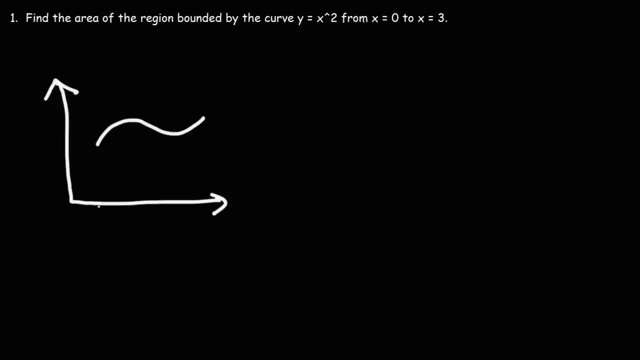 And let's say this is point A and point B, And we want to find the area underneath this curve. In other words, we want to find the area between this curve and the x-axis And let's say this curve is y equals f of x. 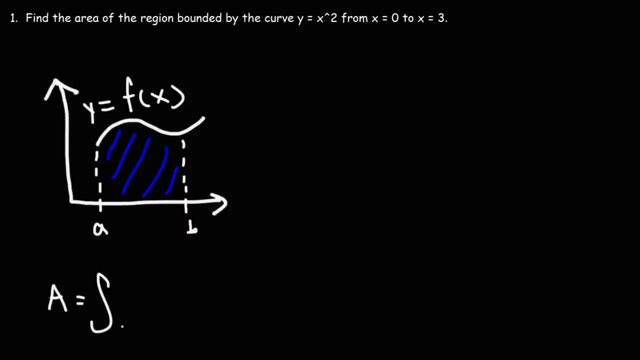 To determine the area under the curve. it's going to be the integral from A to B, Of f, of x, dx. So we just got to find the value of the definite integral from A to B And that's going to give us the area of the region. 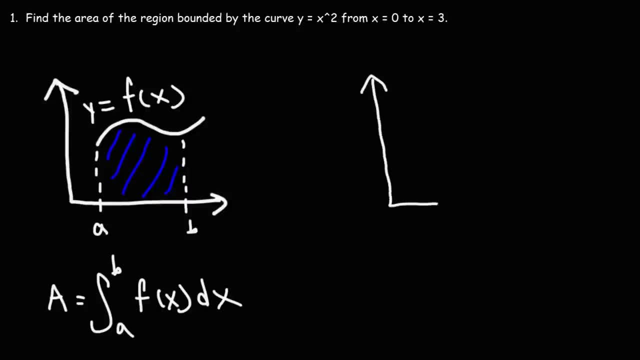 Now you also have this variant of the same formula. So let's say the curve looks like this And we want to calculate the area bounded by the curve, And instead of the x-axis It's going to be the area under the curve. 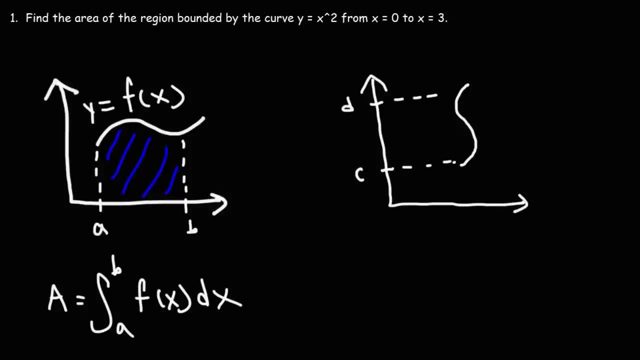 And instead of the x-axis It's going to be with the y-axis. So we want to find the area of this shaded region. In this case, we want this curve to be in terms of y instead of x. So here this is a function of x. 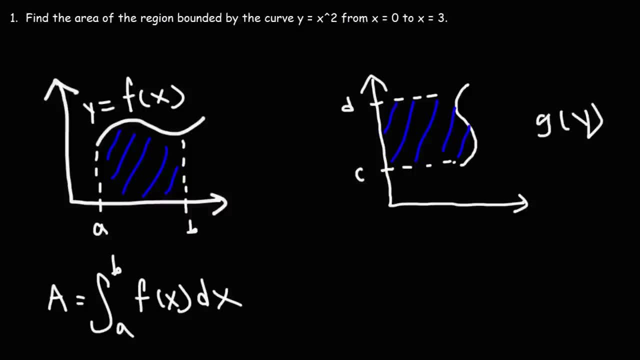 What we need to find is a function of y. Now, y is equal to f of x, So y is a function of x. But in this case, g is a function of x, So g of y is going to equal x. 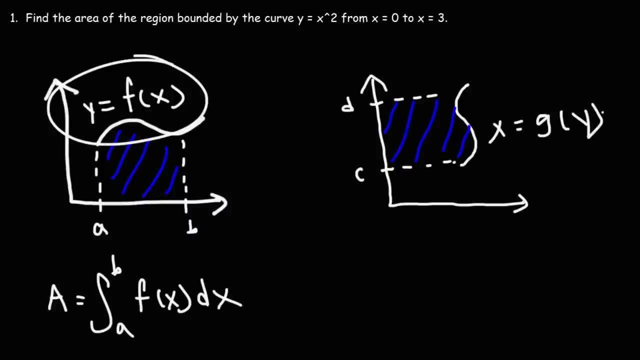 Make sure you see the difference here. Here we have y is equal to f of x. Here we have x is equal to g of y. Now to calculate the area for the second situation, We need to find the definite integral from c to d. 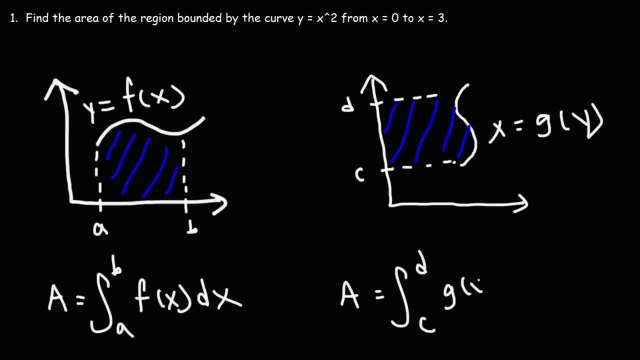 So those are y values of g, of y, dy. So make sure you understand that key difference: A and b are x values, C and d are y values. But for this particular problem We're going to use this form to calculate the area. 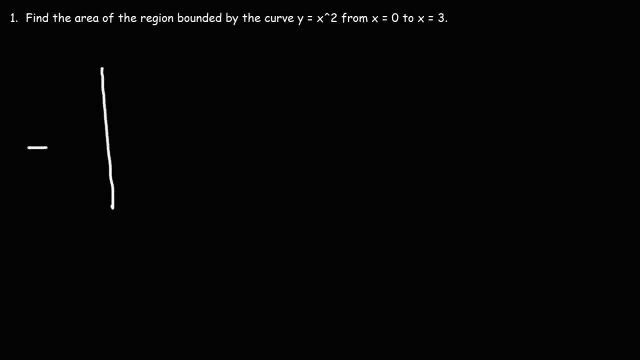 Now the first thing we should do is we should draw a picture. So we have y equals x squared, which looks like this, And we want to find the region bounded by the curve from 0 to 3.. So we only need the right side of that graph. 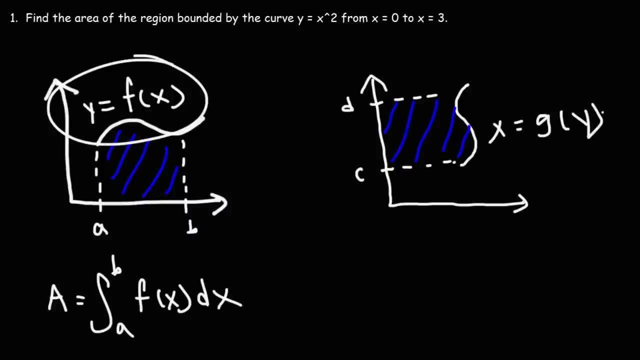 Make sure you see the difference here. Here we have y is equal to f of x. Here we have x is equal to g of y. Now to calculate the area for the second situation, We need to find the definite integral from c to d. 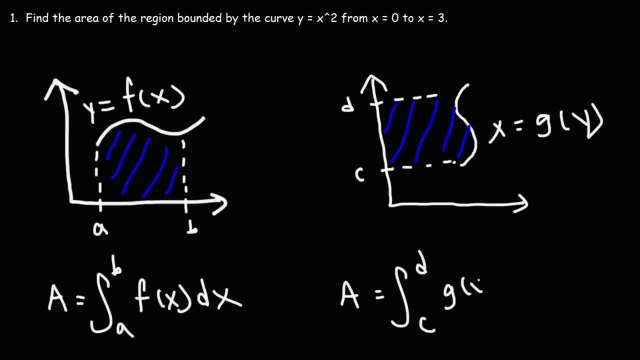 So those are y values of g, of y, dy. So make sure you understand that key difference: A and b are x values, C and d are y values. But for this particular problem We're going to use this form to calculate the area. 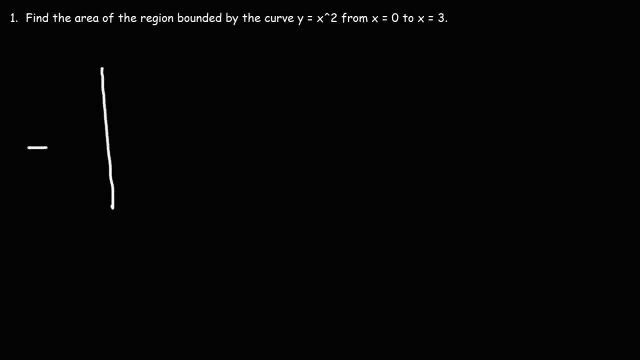 Now the first thing we should do is we should draw a picture. So we have y equals x squared, which looks like this, And we want to find the region bounded by the curve from 0 to 3.. So we only need the right side of that graph. 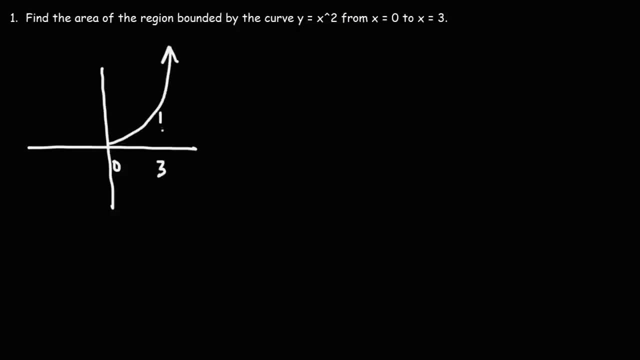 So this is 0. So let's say this point, It's 3.. We're looking for the area of this region here. So, using the formula, The area is going to be the definite integral from a to b of f, of x, dx. 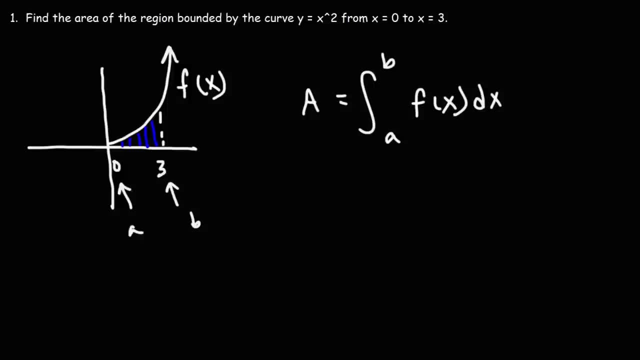 So a is 0.. b is 3.. Those are the limits of integration. And remember, y is equal to f of x And in this problem, y is x squared, So f of x is x squared. Now, using the power rule, the antiderivative of x squared is going to be: 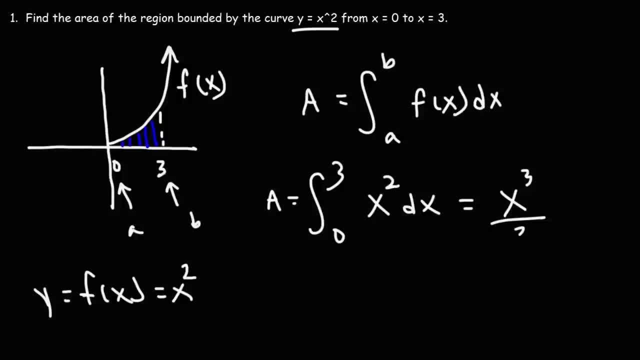 We're going to add 1 to 2.. So we'll get 3.. And then we're going to divide by that result. Now we're going to evaluate it from a to b, from 0 to 3.. So first we're going to plug in 3.. 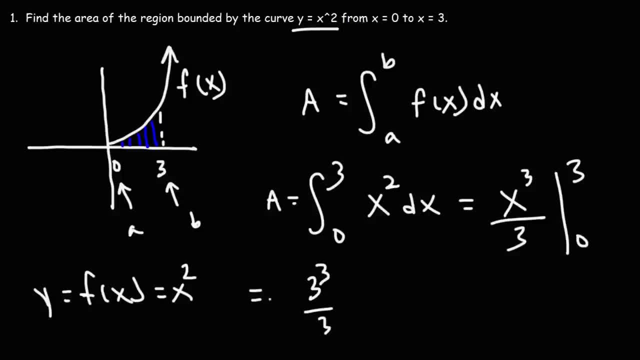 This is going to be 3 to the 3rd over 3.. And then we're going to plug in 0. So it's 0 to the 3rd over 3.. 3 to the 3rd is 27, divided by 3 is 9.. 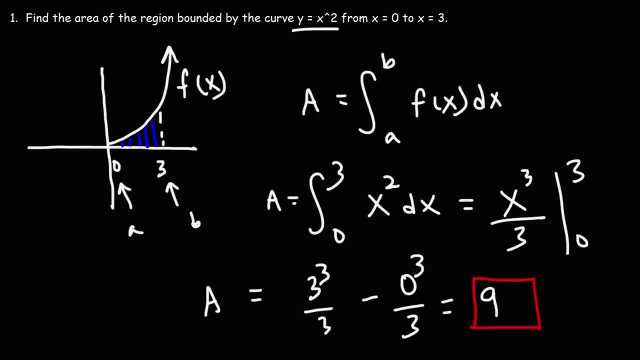 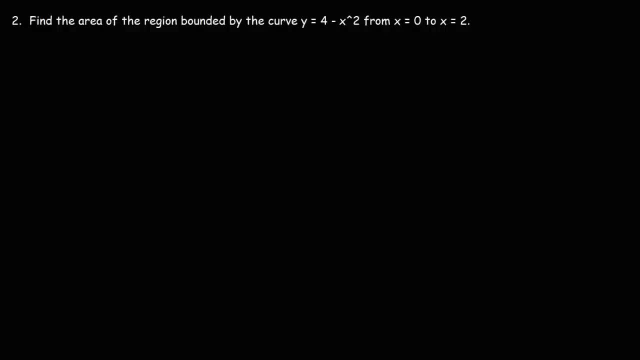 So the area of the region bounded by the curve is equal to 9 square units. Now let's try this problem. Find the area of the region bounded by the curve. Y equals 4 minus x, squared from x equals 0 to x equals 2.. 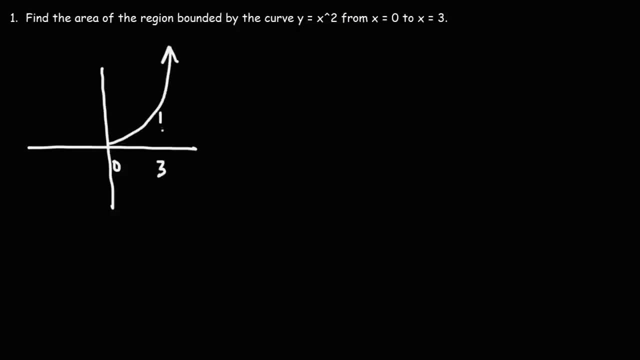 So this is 0. So let's say this point, It's 3.. We're looking for the area of this region here. So, using the formula, The area is going to be the definite integral from a to b of f, of x, dx. 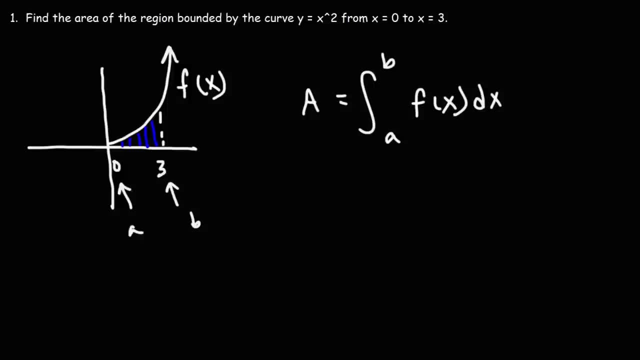 So a is 0.. b is 3.. Those are the limits of integration. And remember, y is equal to f of x And in this problem, y is x squared, So f of x is x squared. Now, using the power rule, the antiderivative of x squared is going to be: 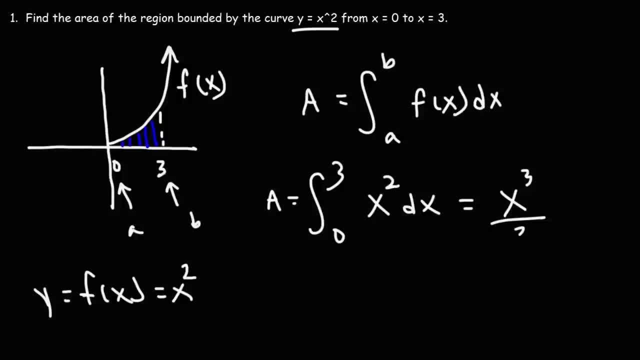 We're going to add 1 to 2.. So we'll get 3.. And then we're going to divide by that result. Now we're going to evaluate it from a to b, from 0 to 3.. So first we're going to plug in 3.. 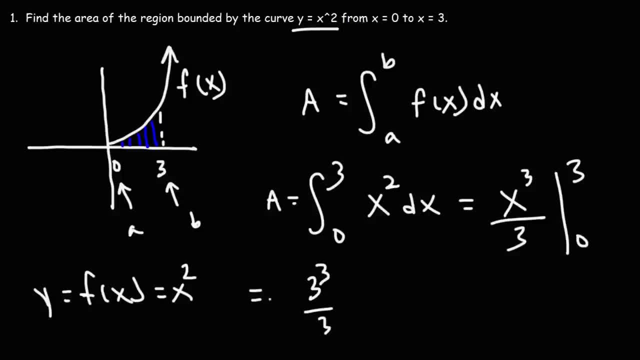 This is going to be 3 to the 3rd over 3.. And then we're going to plug in 0. So it's 0 to the 3rd over 3.. 3 to the 3rd is 27, divided by 3 is 9.. 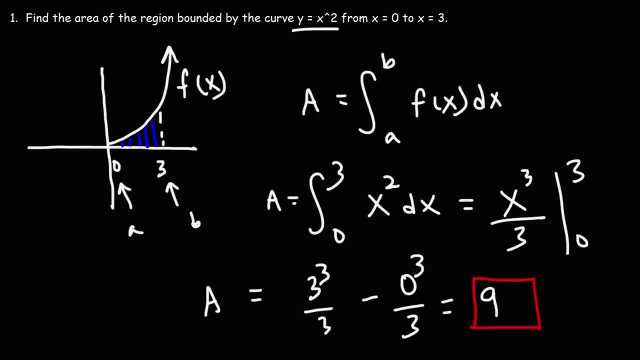 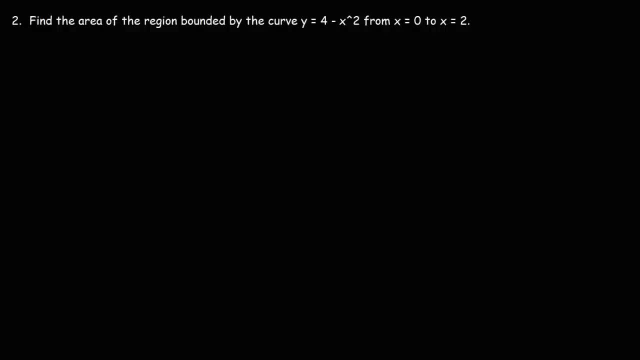 So the area of the region bounded by the curve is equal to 9 square units. Now let's try this problem. Find the area of the region bounded by the curve. Y equals 4 minus x, squared from x equals 0 to x equals 2.. 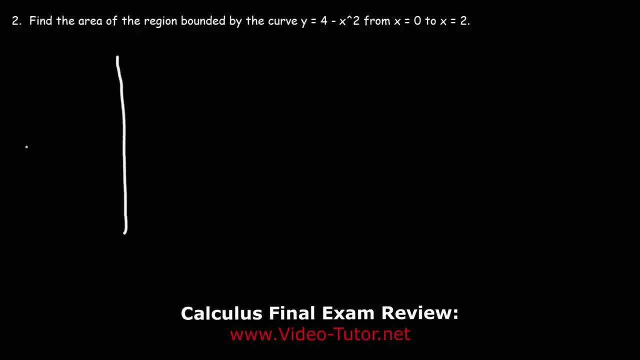 So let's begin by drawing a picture. Now we know that positive x squared looks like this: Negative x squared is a parabola that opens downward Now that parabola is shifted 4 units up. So instead of starting from the origin, it's going to start 4 units above that. 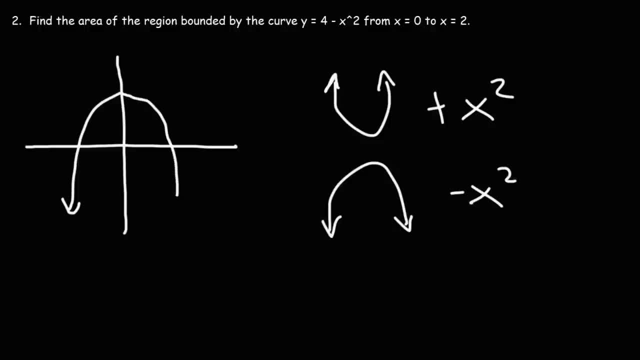 So our graph is going to look like this. Now it's always good to find the x-intercepts. To find the x-intercept, set y equal to 0 and solve for x. So what we have is the difference of perfect square. 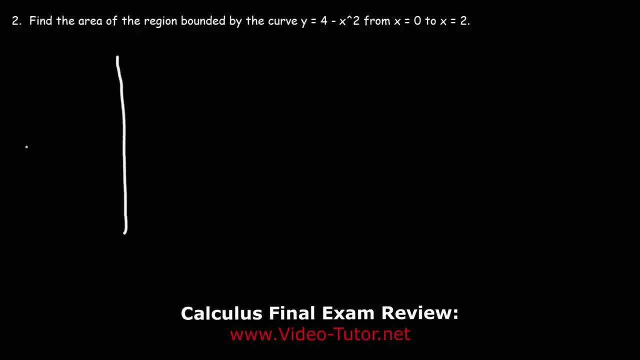 So let's begin by drawing a picture. Now we know that positive x squared looks like this: Negative x squared is a parabola that opens downward Now that parabola is shifted 4 units up. So instead of starting from the origin, it's going to start 4 units above that. 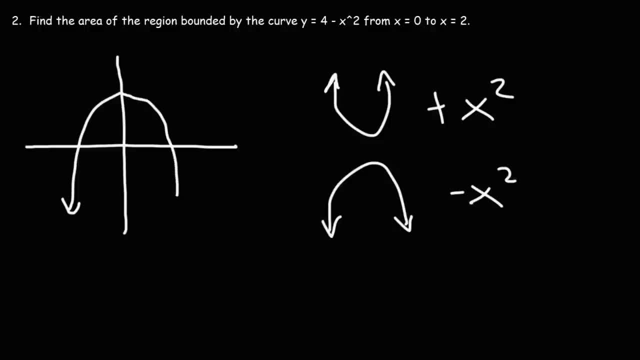 So our graph is going to look like this. Now it's always good to find the x-intercepts. To find the x-intercept, set y equal to 0 and solve for x. So what we have is the difference of perfect square. 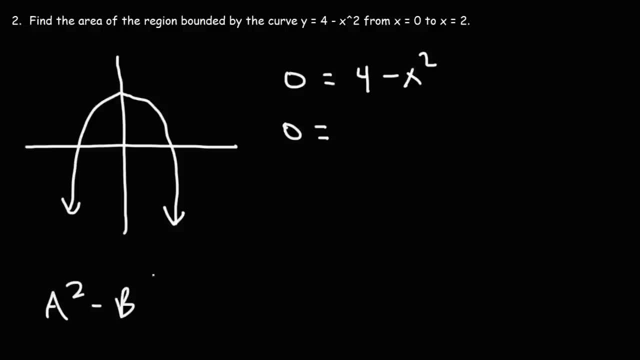 So we could use the formula a squared minus b squared to factor it into a plus b times a minus b. So the square root of 4 is 2.. And the square root of x squared is x. So this is going to be 2 plus x and 2 minus x. 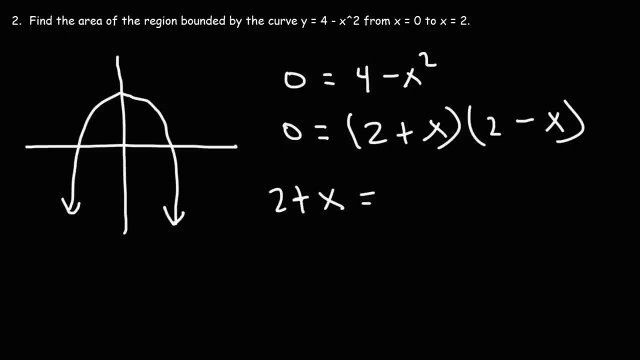 If you set the first factor equal to 0,, you're going to get x is equal to negative 2.. And if you set the second factor equal to 0, and if you solve for x, you'll get x is equal to positive 2.. 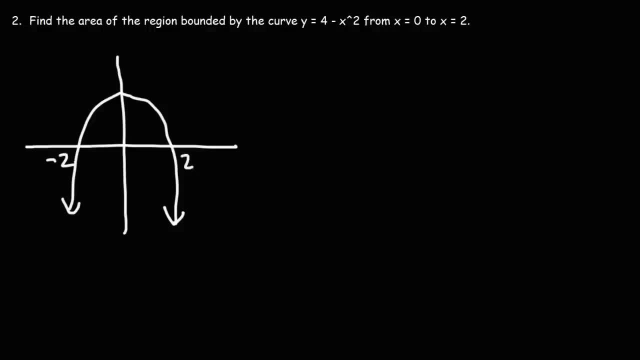 So this intercept is at negative 2.. This one is at positive 2.. Now we want to find the area of the region bounded by the curve from 0 to positive 2. So only just the right side of this graph. So using the formula, the area is the definite integral from a to b, of f, of x, dx. 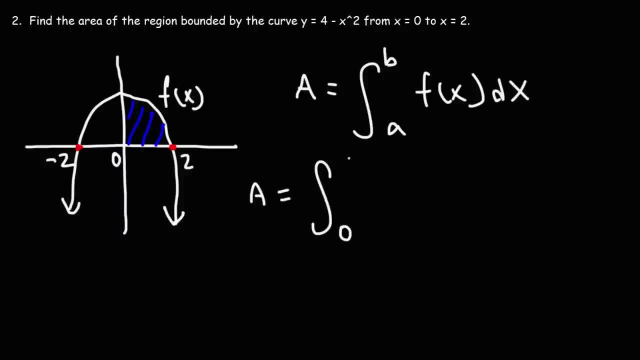 We have that the area is going to be the integral from 0 to 2.. And f of x is y, so that is 4 minus x squared and then dx. Now the antiderivative of the constant 4 is simply just 4x. 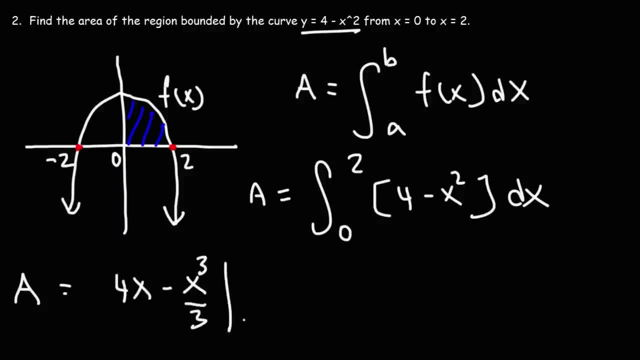 For x squared. we know it's x cubed over 3. And we're going to evaluate it from 0 to 2.. So first we're going to plug in 2.. So this is 4 times 2 minus 2 to the third over 3.. 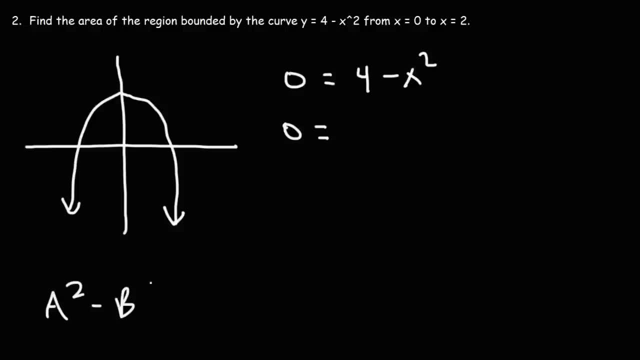 So what we have is the difference of perfect square. So what we have is the difference of perfect square. So we could use the formula a squared minus b squared to factor it into a plus b times a minus b. So the square root of 4 is 2.. 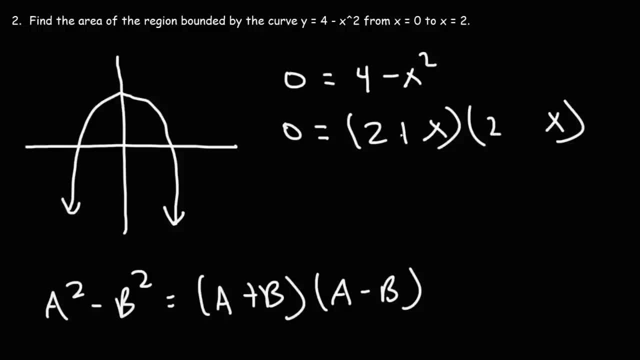 And the square root of x squared is x. So this is going to be 2 plus x and 2 minus x. If you set the first factor equal to 0,, you're going to get x is equal to negative 2.. And if you set the second factor equal to 0, and if you solve for x, you'll get x is equal to positive 2.. 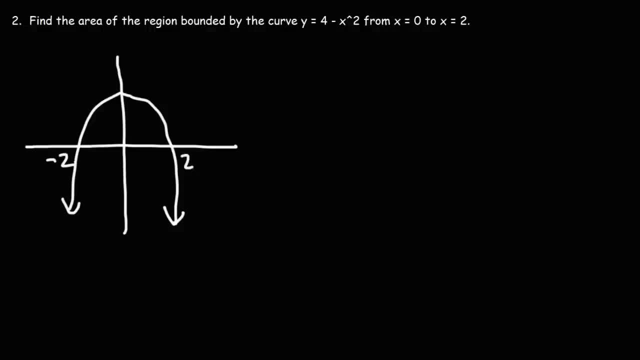 So this intercept is at negative 2.. This one is at positive 2.. Now we want to find the area of the region bounded by the curve from 0 to positive 2. So only just the right side of this graph. So using the formula, the area is the definite integral from a to b, of f, of x, dx. 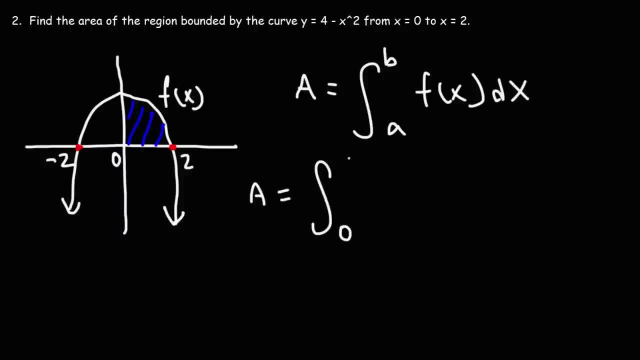 We have that the area is going to be the integral from 0 to 2.. And f of x is y, so that is 4 minus x squared and then dx. Now the antiderivative of the constant 4 is simply just 4x. 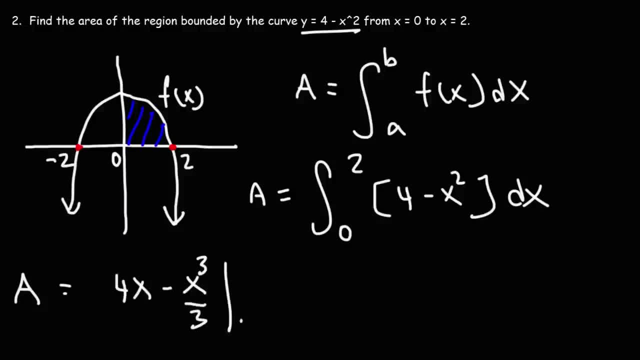 For x squared. we know it's x cubed over 3. And we're going to use that as the derivative of the constant 4.. So we're going to evaluate it from 0 to 2.. So first we're going to plug in 2.. 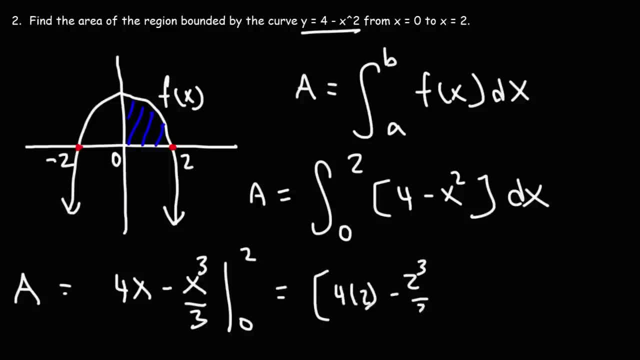 So this is 4 times 2 minus 2 to the 3rd over 3.. And then we'll plug in 0.. So 4 times 0 minus 0 to the 3rd over 3.. 4 times 2 is 8.. 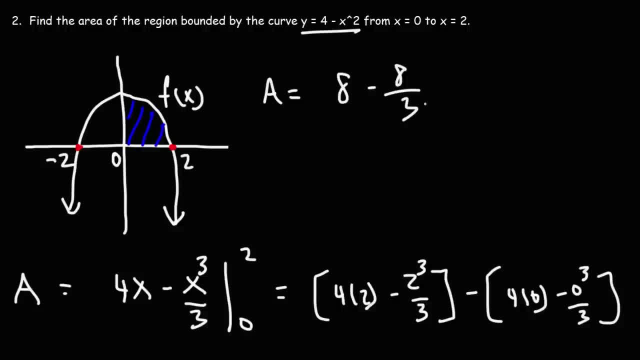 2 to the 3rd power, 2 times 2 times 2, that's 8 as well, And everything here is simply 0.. Now, in order to combine these two numbers, we have a fraction and a whole number. 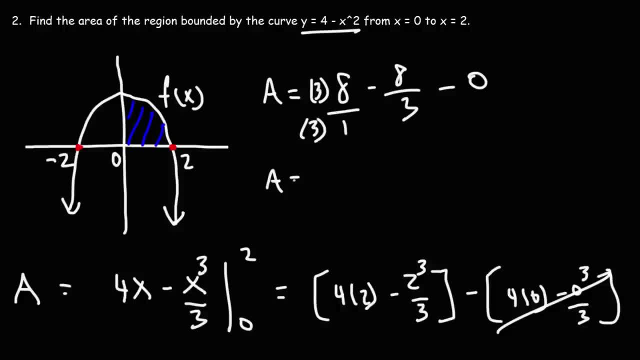 we need to get common denominators. So I'm going to multiply 8 by 3 over 3.. So this is going to be 24 over 3, minus 8 over 3.. 24 minus 8 is 16.. So the area of the shaded region is going to be 16 over 3 square units. 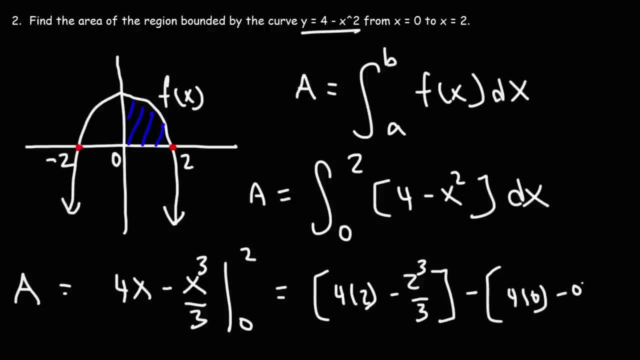 And then we'll plug in 0. So 4 times 0 minus 0 to the third over 3.. 4 times 2 is 8.. 2 to the third power 2 times 2 times 2, that's 8 as well. 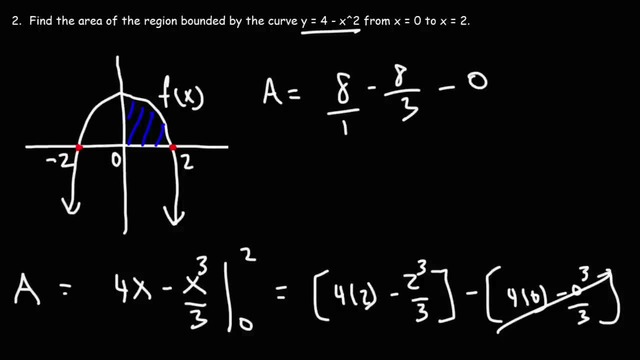 And everything here is simply 0.. Now, in order to combine these two numbers- we have a fraction and a whole number- We need to get common denominators. So I'm going to multiply 8 by 3 over 3.. So this is going to be 24 over 3, minus 8 over 3.. 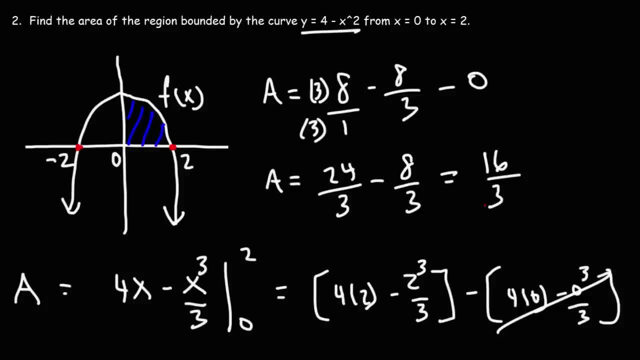 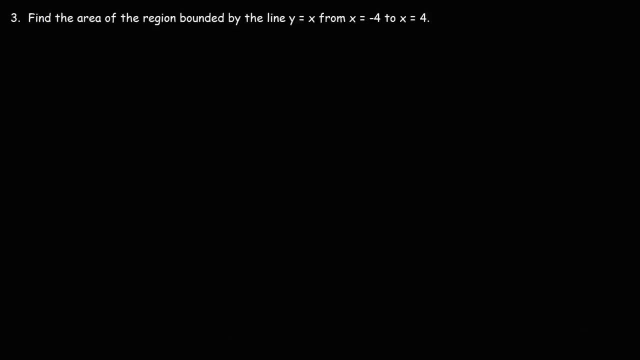 24 minus 8 is 16.. So the area of the shaded region is going to be 16 over 3 square units. Now let's move on to number 3.. Find the area of the region bounded by the line y equals x. from x equals negative 4 to x equals 4.. 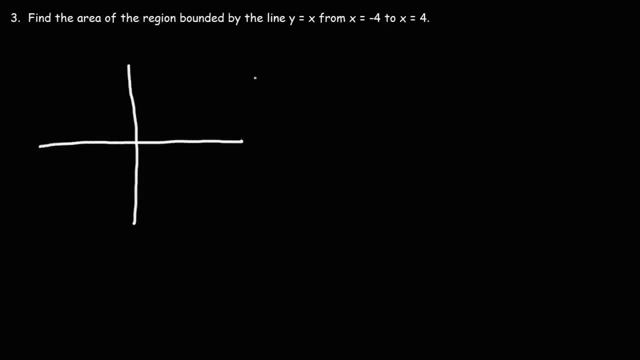 So let's start with a picture, And here is the line: y equals x, or at least a rough sketch of it. Somewhere over here it's going to be negative 4.. And somewhere over here we have positive 4.. 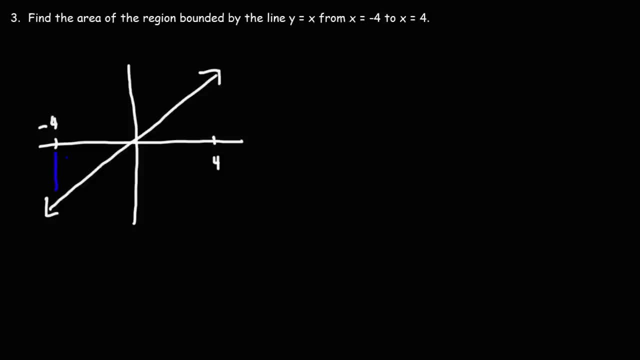 So we want to find the area of these two shaded regions Now. it's important to understand that if you take the indefinite integral from negative 4 to 4, if you integrate it, you're going to get a value of 0.. 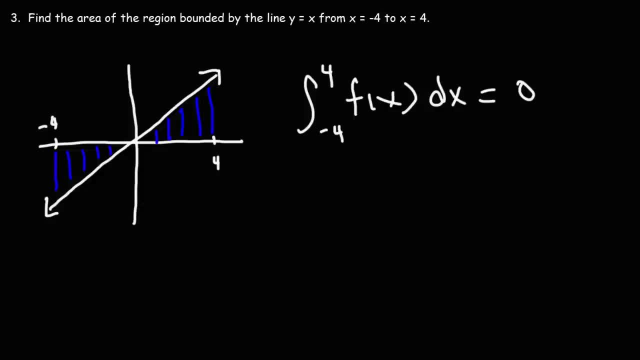 The area on the right. this is going to be a positive value because it's above the x-axis, The area on the left is going to be a positive value And the area on the right is going to be a negative value because it's above the x-axis. 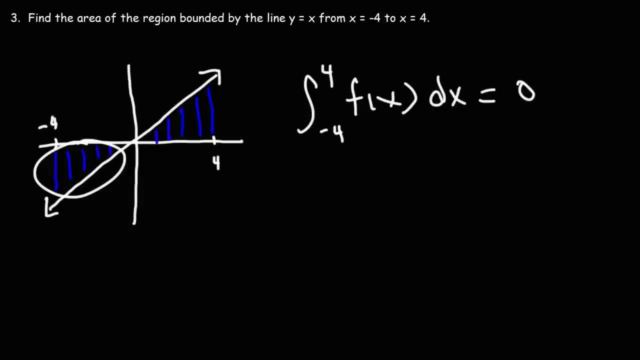 So we're going to find the area of these two shaded regions left that you'll get will be a negative value because it's below the x-axis. Now, typically when you're solving problems like this, if it tells you to find the area you typically want, 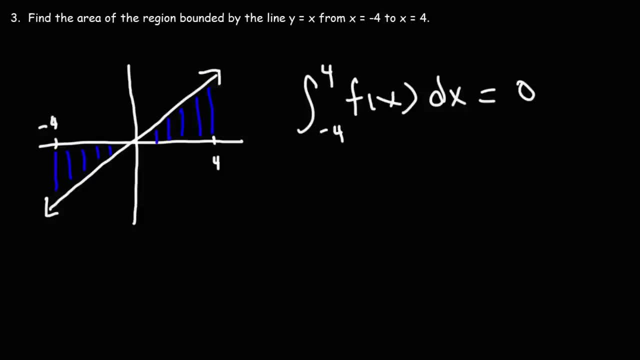 a positive value. Now there's two ways in which we could do this. We could basically take this side and multiply it by two, or we could break this up into two separate integrals. This one will be positive, but this one, we can add a negative sign to it to make it positive. 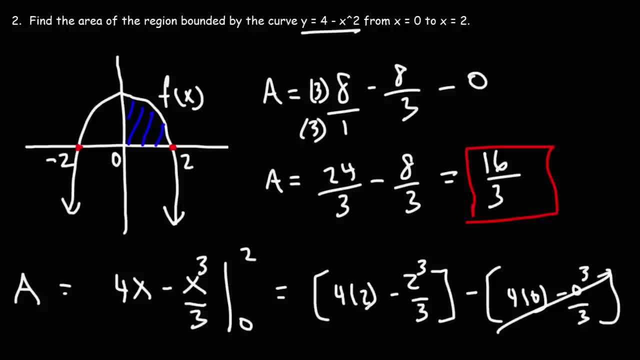 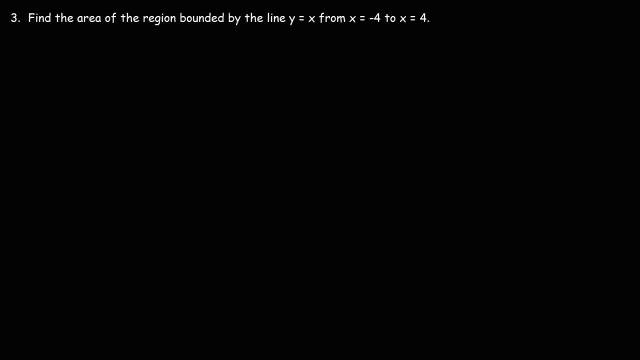 Thanks for watching. Now let's move on to number 3. Find the area of the region bounded by the line y equals x, from x equals negative 4 to x equals 4.. So let's start with a picture, And here is the line y equals x, or at least a rough sketch of it. 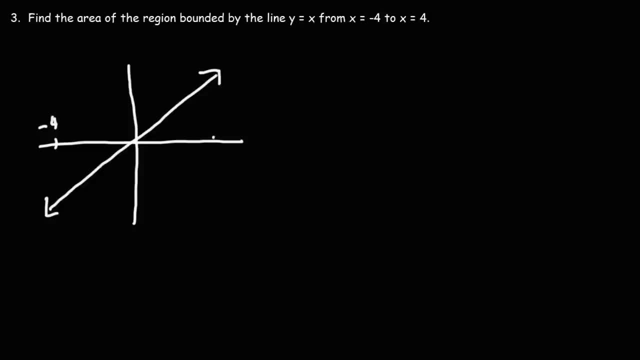 Somewhere over here it's going to be negative 4.. And somewhere over here we have positive 4.. So we want to find the area of the region bounded by the line y equals x. So we want to find the area of these two shaded regions. 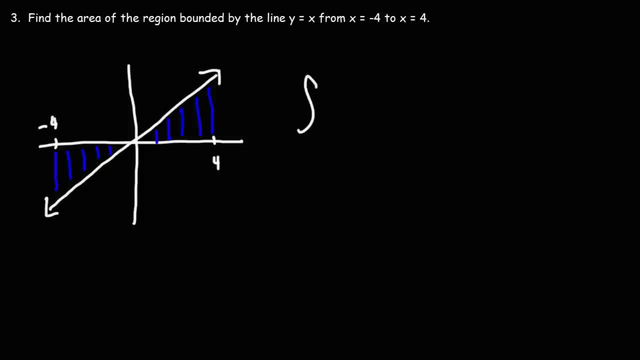 Now it's important to understand that if you take the indefinite integral from negative 4 to 4, if you integrate it, you're going to get a value of 0.. The area on the right: this is going to be a positive value because it's above the x-axis. 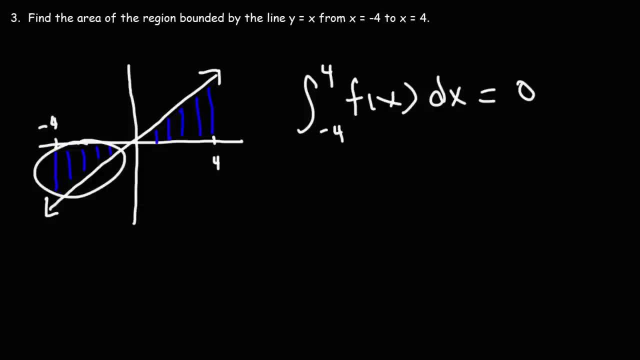 The area on the left that you'll get will be a negative value because it's above the x-axis. So we want to find the area of these two shaded regions Because it's below the x-axis. Now, typically when you're solving problems like this, if it tells you to find the area, 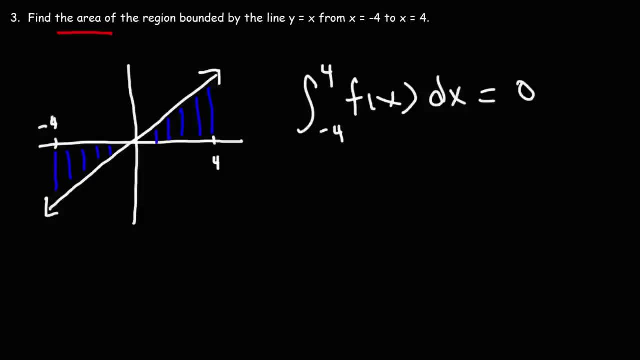 you typically want a positive value. Now, there's two ways in which we could do this. We could basically take this side and multiply it by 2. Or we could break this up into two separate integrals. This one will be positive, but this one, we can add a negative sign to it to make it positive. 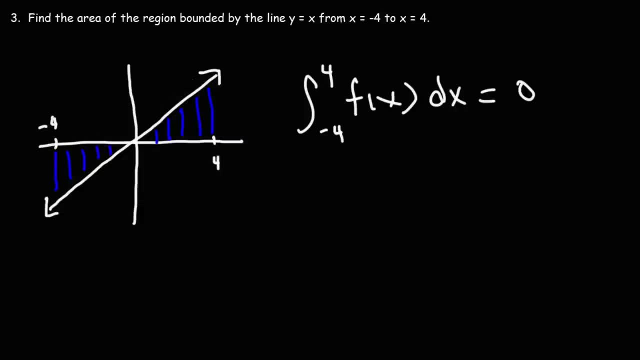 But due to symmetry, we can say that the area is simply going to be twice the value of the right side. So if we integrate it from 0 to 4, and then simply double our answer, we're going to get the area of the shaded region. 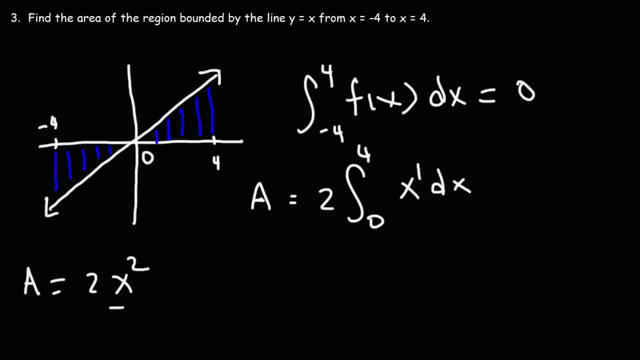 So the antiderivative of x is going to be x squared over 2.. And if we integrate it from 0 to 4, I mean evaluate it from 0 to 4, the 2s will cancel. So we just have x squared from 0 to 4.. 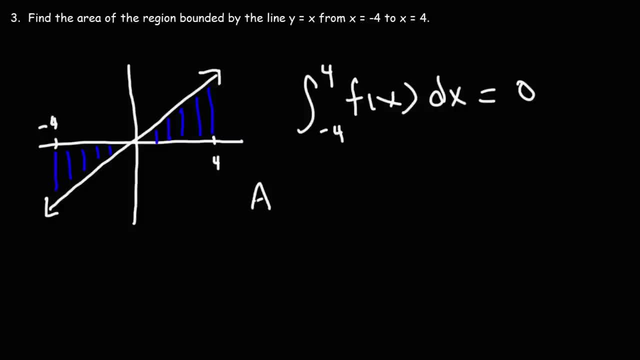 But due to symmetry, we can say that the area is simply going to be twice the value of the right side. So if we integrate it from zero to four and then simply double our answer, we're going to get the area of the curve, or I mean the area of the shaded region. 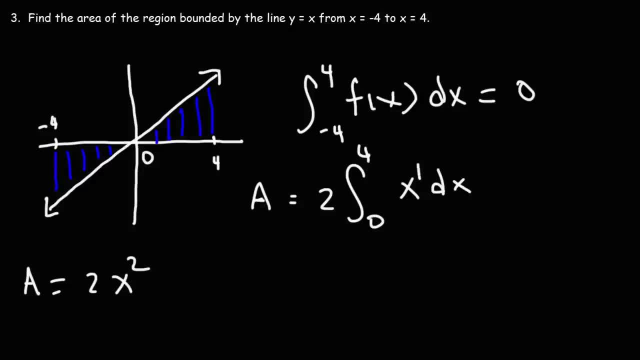 So the anti-derivative of x is going to be x squared over two, and if we integrate it from zero to four- I mean evaluate it from zero to four- the twos will cancel. So we just have x squared from zero to four and if we plug in four, this is going to be four squared, and if we plug in zero. 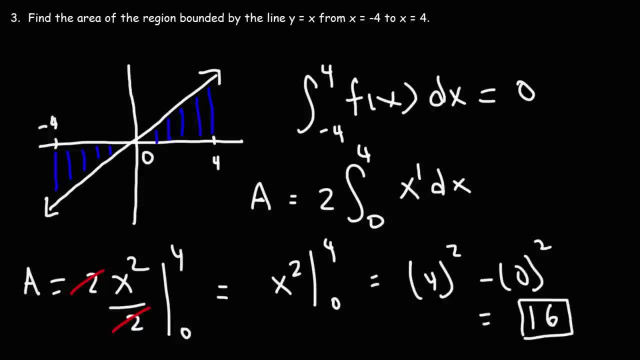 and we're going to get 16 in total. So that is the area of these two shaded regions. It's 16 square units. Now, we could confirm this answer using geometry, So let's focus on the top right part. What we have is a triangle, The base. 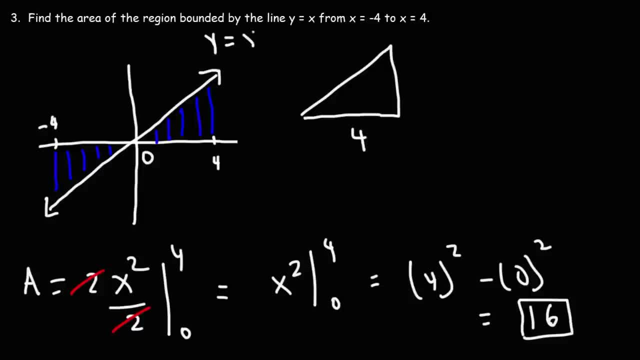 of the triangle is four. Now the equation is: y is equal to x. So when x is four, y is four, Which means this triangle has a height of four. Now the area of a triangle is one half base times height, So one half four times four. 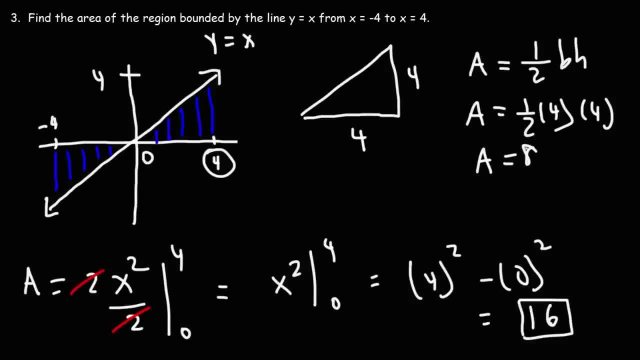 Four times four is 16.. Half of that is eight. So the area of this triangle is eight and the area of the other triangle is also eight. When you add the two together, you get 16.. So be careful with problems where you're dealing with negative areas or 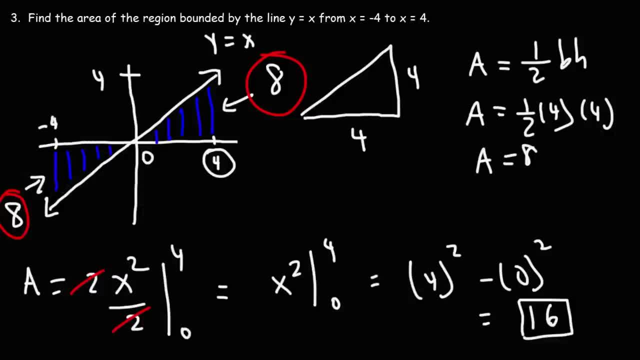 where the region is below the x-axis. If you have a symmetrical situation like this, you could just calculate the area of the right side and multiply by two. that will give you the entire answer. In other cases, if you don't have symmetry, 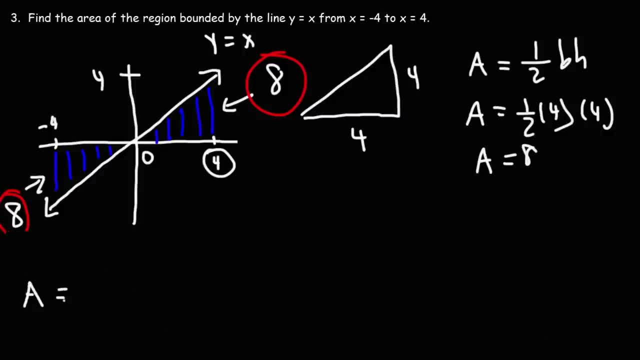 you need to do it this way. So the area will be the integral from zero to four x dx. That will give us the area of the right side and then minus the integral from negative 4 to 0, x dx. So this part will give us a negative area times negative 1.. That'll make 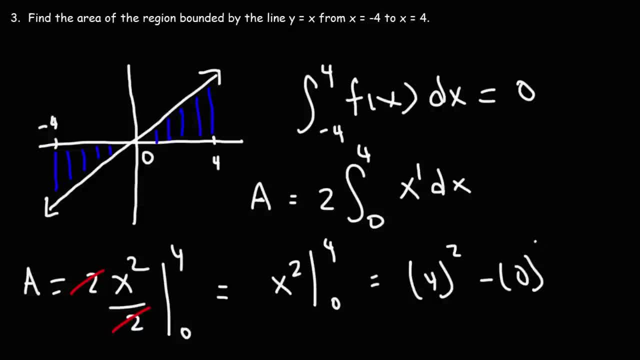 And if we plug in 4, this is going to be 4 squared. And if we plug in 0, then we're going to get 16 in total. So that is the area of these two shaded regions. It's 16 square units. 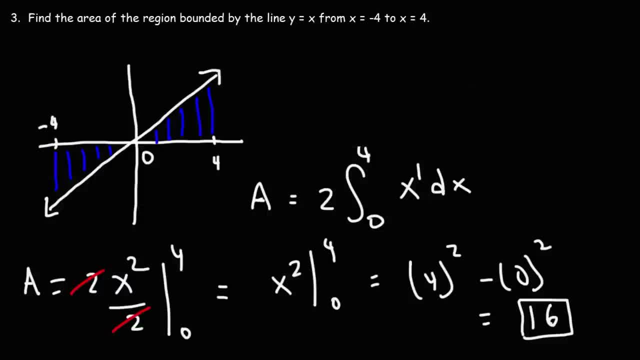 Now we could confirm this answer using geometry. So let's focus on the top right part. What we have is a triangle. The base of the triangle is 4.. Now the equation is y is equal to x. So when x is 4, y is 4,, which means this triangle has a height of 4.. 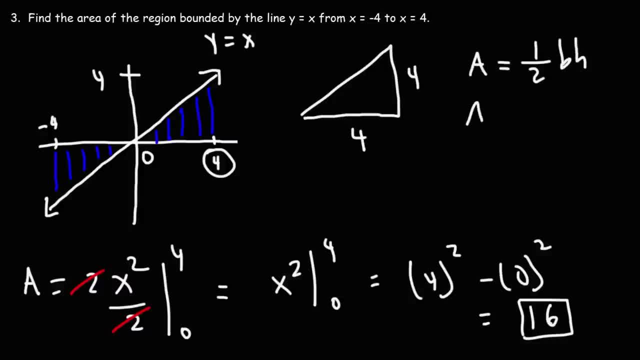 Now the area of a triangle is 1 half base times height, So 1 half 4 times 4.. 4 times 4 is 16.. Half of that is 8.. So the area of this triangle is 8.. 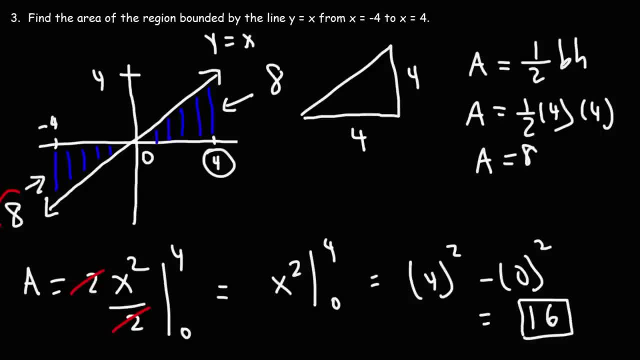 And the area of the other triangle is also 8.. When you add the two together, you get 16.. So be careful with problems where you're dealing with negative areas or where the region is below the x-axis. If you have a symmetrical situation like this, 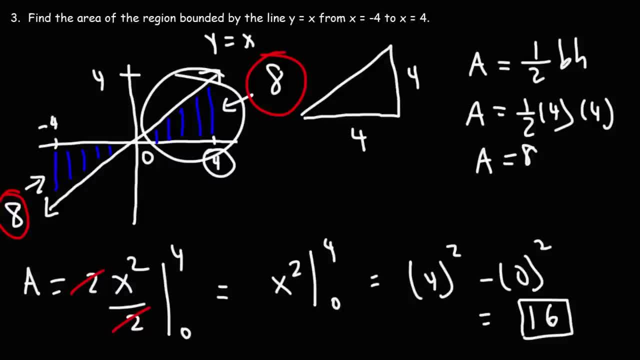 you could just calculate the area of the right side and multiply it by 2.. That will give you the entire answer. In other cases, if you don't have symmetry, you need to do it this way. So the area will be the integral from 0 to 4, x, dx. 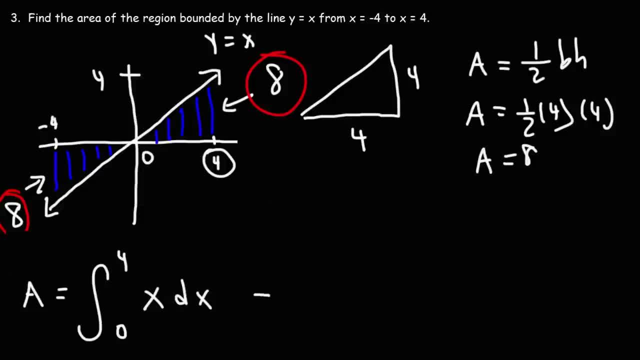 That will give us the area of the right side And then minus the integral from negative 4 to 0,, x, dx. So This part will give us a negative area times negative 1. That will make this positive 8. And will help us get the right answer. 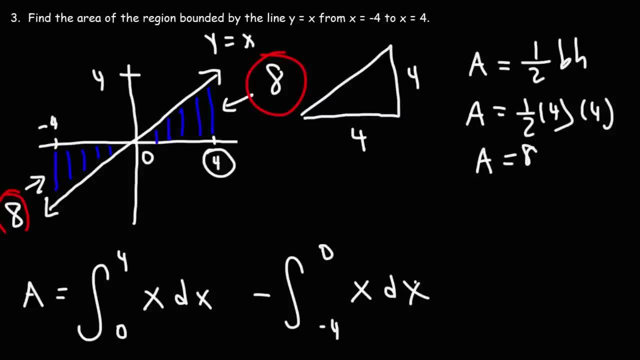 So that's how you can calculate the total area of the region, bottom line of the curve. For regions that are above the x-axis, you can put a positive sign. For regions that are below the x-axis, add a negative sign to it. 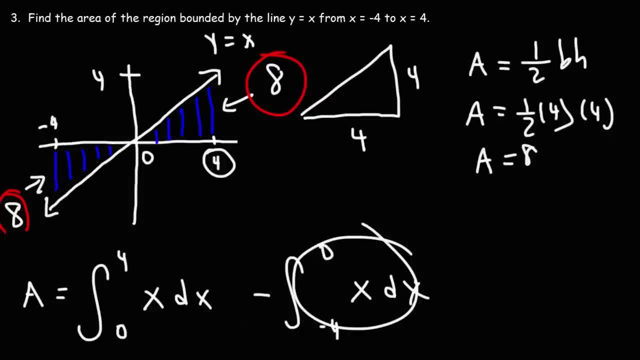 this positive 8 and will help us get the right answer. So that's how you can calculate the total area of the region, bottom line of the curve For regions that are above the x-axis. you can put a positive sign. For regions that are below the x-axis, add a negative sign to it so that your 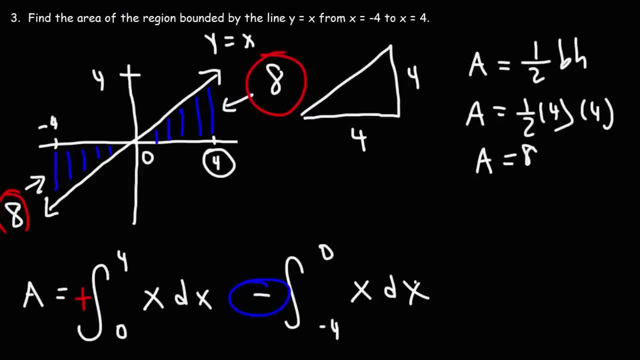 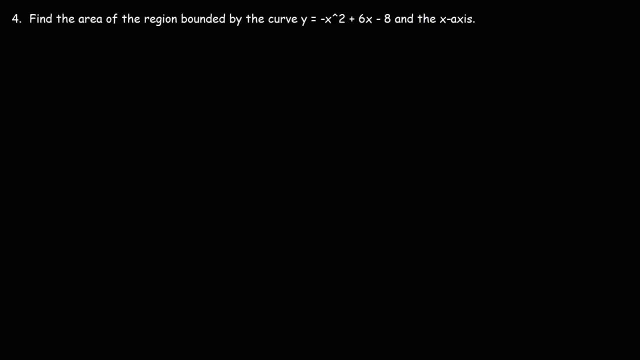 overall answer will be positive. Number 4, find the area of the region bounded by the curve y, equal, negative x squared plus 6x, minus 8, and the x-axis. So what we have here is a quadratic equation, and whenever you have it in standard form, it's good to find the x-intercepts. 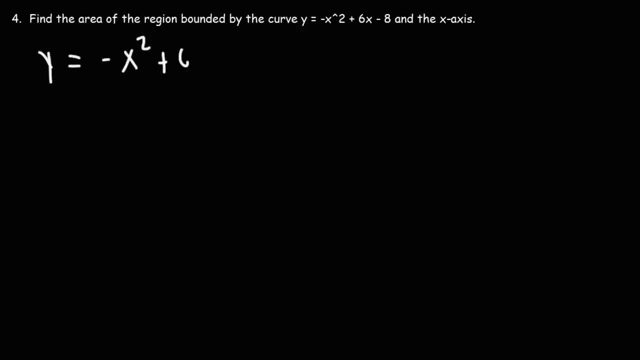 So right now it's negative x squared plus 6x minus 8.. So to find the x-intercepts we need to replace y with 0.. Now I'm going to factor out a negative 1.. So this becomes x squared minus 6x. 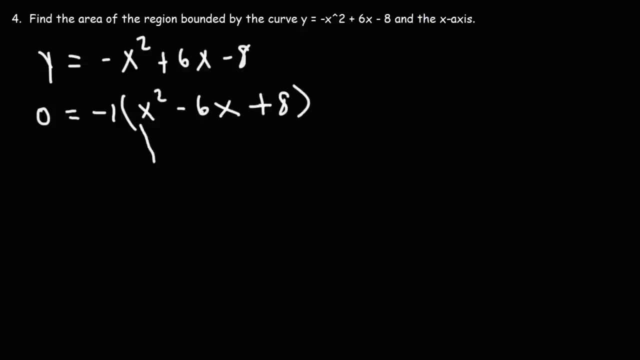 plus 8. So we have a trinomial where the leading coefficient is 1. So to factor it we need to find two numbers that multiply to 8 but add to the middle coefficient negative 6. So those two numbers add up to negative 4.. Negative 2 plus negative 4 adds up to negative 6, but negative 2 times negative 4. 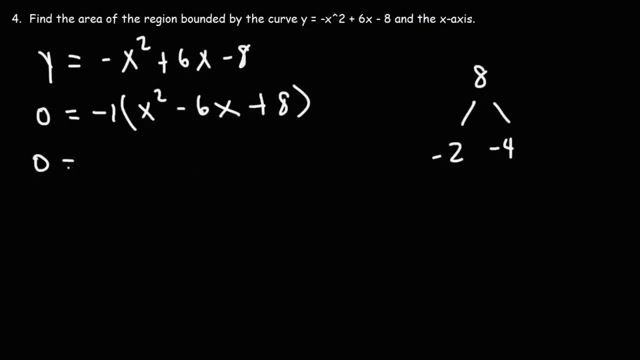 multiplies to positive 8. So to factor this expression, it's going to be x minus 2 times x minus 4.. Using the zero product property, if we set each factor equal to 0, we'll get the two intercepts. 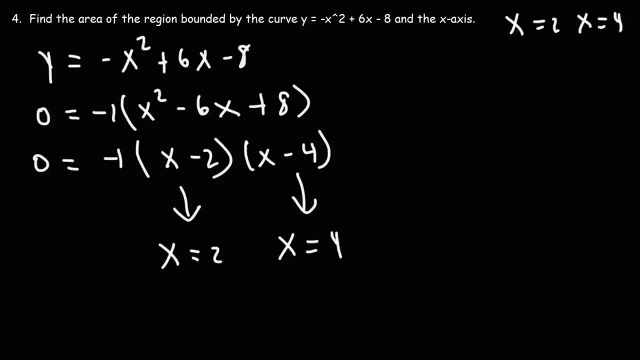 x equals 2 and x equals 4, which I'm going to rewrite it here. Now notice that we have a parabola, but with a negative in front of the x squared term. So that means that the parabola is going to open downward. With this information, we can draw: 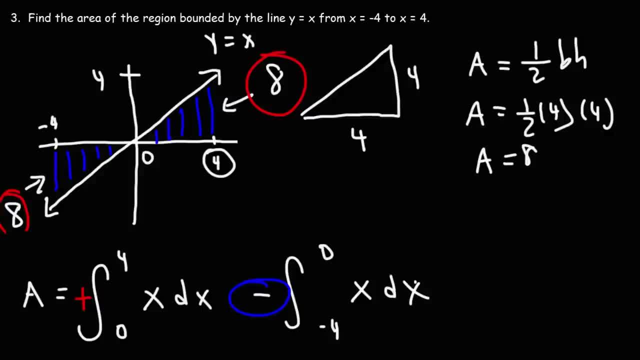 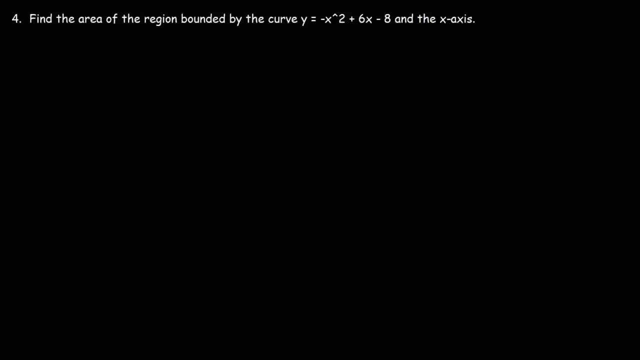 So that your overall answer will be positive. Number 4. Find the area of the region bounded by the curve y, equal, negative x squared plus 6x, minus 8, and the x-axis. So what we have here is a quadratic equation And whenever you have it in standard form, 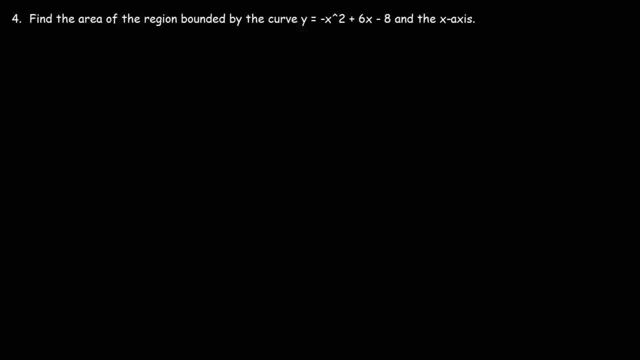 it's good to find the x-intercepts. So right now it's negative x squared plus 6x minus 8.. So to find the x-intercepts we need to replace y with 0.. Now I'm going to factor out a negative 1.. 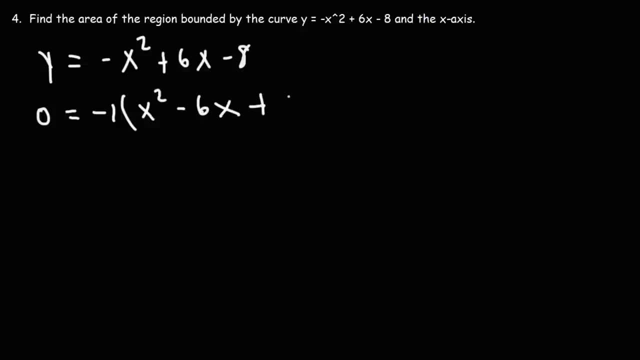 So this becomes x squared minus 6x plus 8.. So we have a trinomial where the leading coefficient is 1. So to factor it, we need to find two numbers that multiply to 8 but add to the middle coefficient negative 6.. 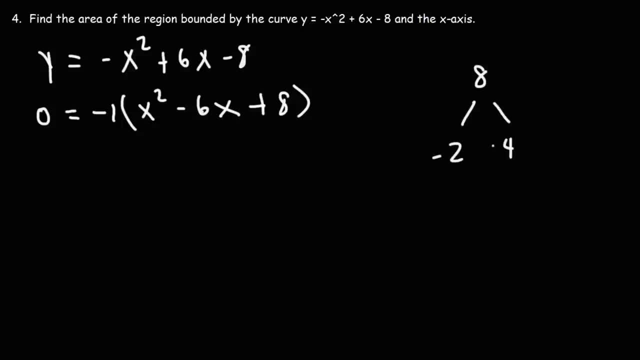 So those two numbers will be negative 2 and negative 4.. Negative 2 plus negative 4 adds up to negative 6, but negative 2 times negative 4.. 4 multiplies to positive 8.. So to factor this expression, it's going to be: 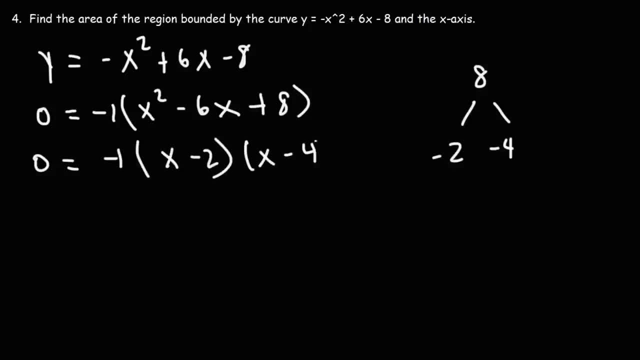 x minus 2 times x minus 4.. Using the zero product property, if we set each factor equal to 0, we'll get the two intercepts x equals 2 and x equals 4, which I'm going to rewrite it here. 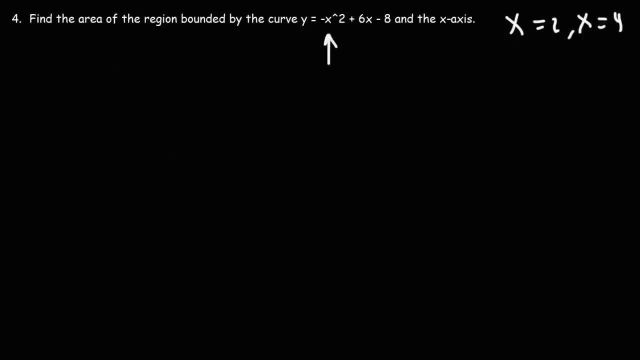 Now notice that we have a negative 4, and we have a parabola, but with a negative in front of the x squared term. So that means that the parabola is going to open downward. With this information we can draw a rough sketch, accurate enough. 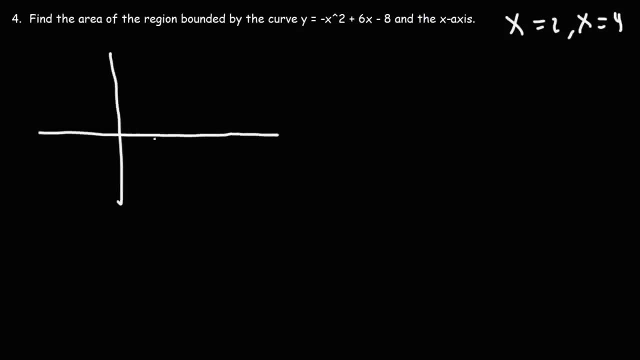 that will help us to get the right answer. So we have an intercept at 2 and another one at 4.. And the graph shows that the intercept at 2 is equal to the intercept at 4.. So we have an intercept at 2 and another one at 4.. 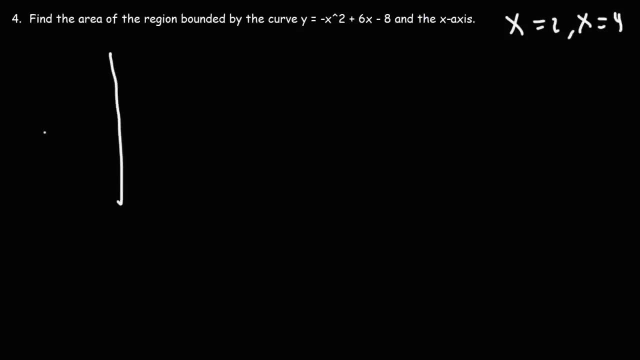 a rough sketch, accurate enough that will help us to get the right answer. So we have an intercept at 2 and another one at 4.. And the graph will look something like this- Let me use a different color. So the region bounded by the curve and the x-axis has to be none other than this region here. 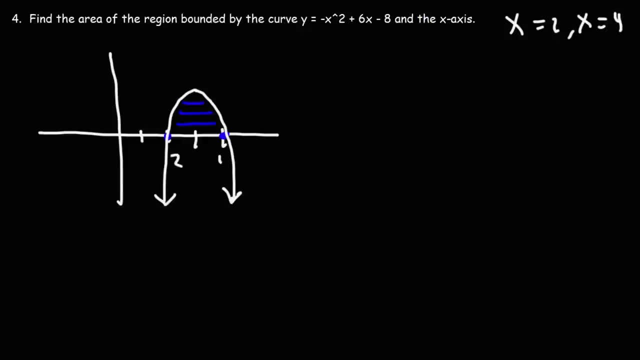 So we need to integrate it from 2 to 4, from one x-intercept to the other x-intercept. So the area is going to be the definite integral, from 2 to 4, of the original expression negative x squared plus 6x minus 8.. 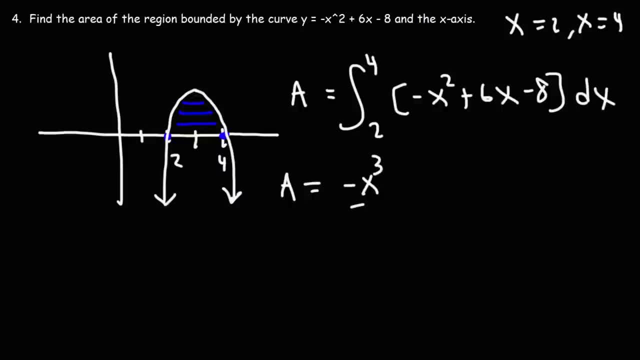 So the antiderivative of x squared is going to be x cubed over 3.. For x, it will simply be x squared over 2. And for a constant we just need to add an x to it. So just to simplify this expression, we have negative: 1 over 3, x cubed, and 6 over 2 is 3.. 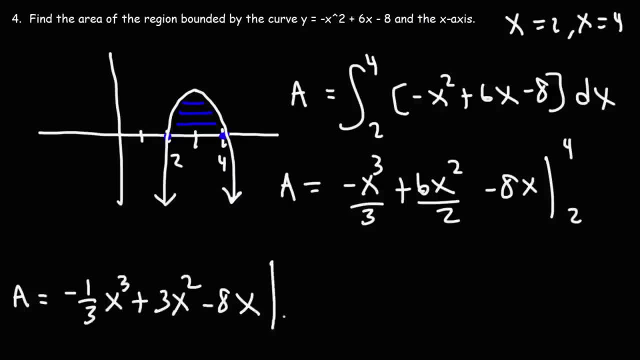 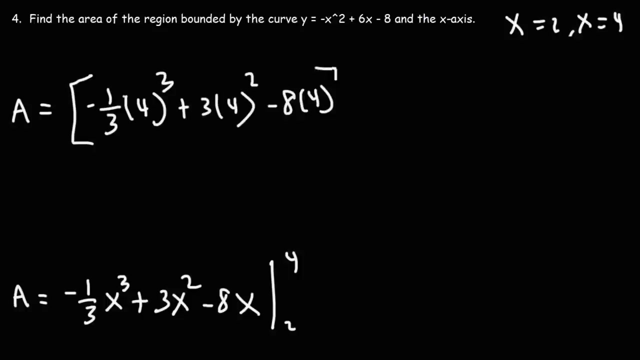 So this is plus 3x squared and then minus 8x evaluated from 2 to 4.. So let's begin by plugging in 4. And then minus. Now let's use the lower limit of integration. Let's plug in 2.. 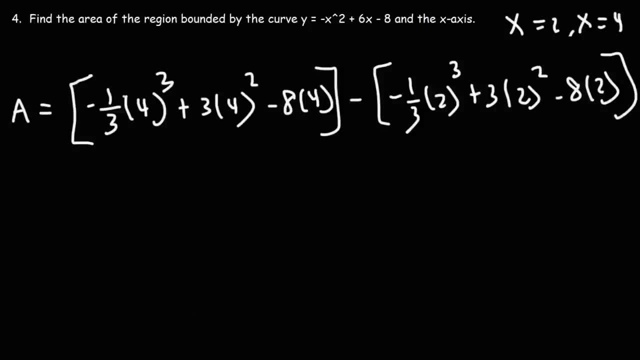 And now, at this point we just got to do the math. So 4 cubed is 64,. 4 squared is 16 times 3,, that's 48,. 8 times 4 is 32,. 2 to the 3rd is 8,. 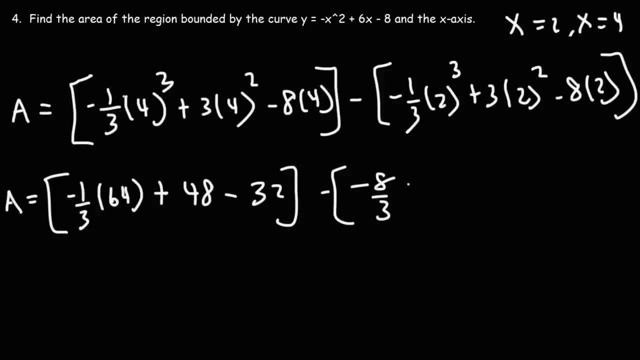 so this becomes negative. 8 over 3, 2 squared is 4 times 3 is 12, 8 times 2 is 16.. So right now we have negative 64 over 3,, 48 minus 32,, that's positive 16,. 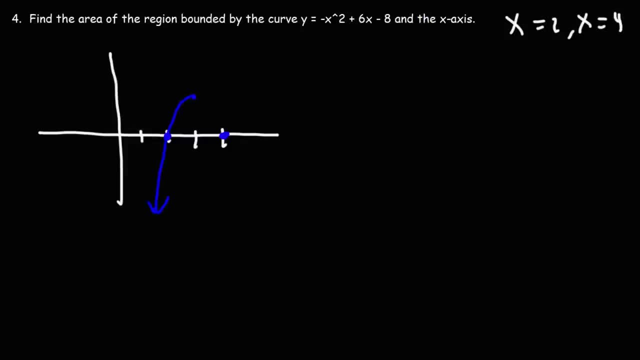 And the graph will look something like this- Let me use a different color. So the region bounded by the curve and the x-axis has to be none other than this region here. So we need to integrate it from 2 to 4.. From one x-intercept. 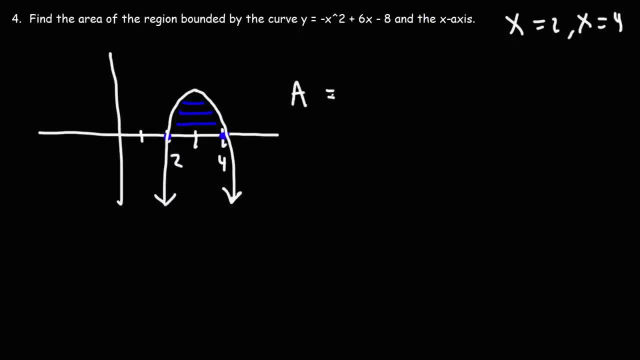 to the other x-intercept. So the area is going to be the definite integral from 2 to 4 of the original expression negative x squared plus 6x minus 8.. So the antiderivative of x squared is going to be x cubed over 3.. 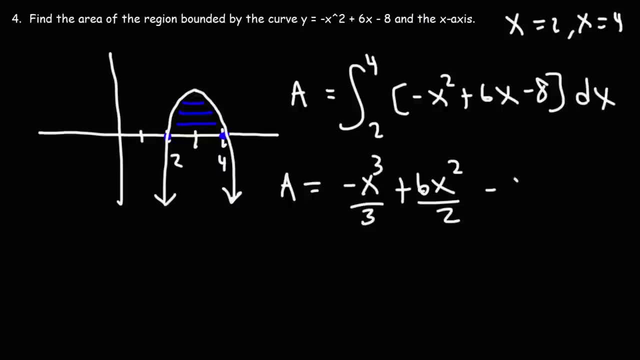 For x, it will simply be x squared over 2. And for a constant, we just need to add an x to it. So just to give you an idea, just to simplify this expression, we have negative 1 over 3, x cubed. 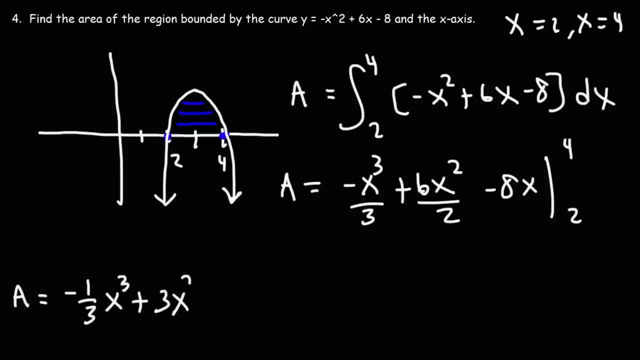 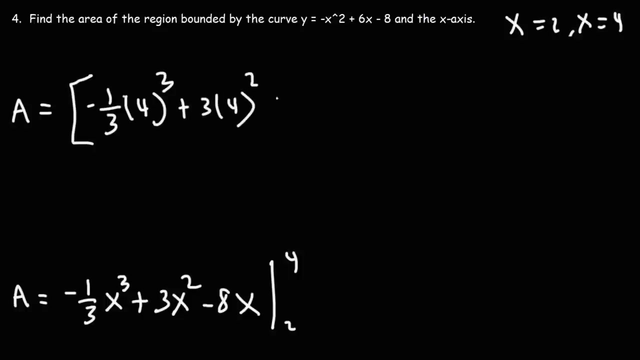 and 6 over 2 is 3.. So this is plus 3x squared and then minus 8x evaluated from 2 to 4.. So let's begin by plugging in 4. And then minus. Now let's use the lower limit of integration. 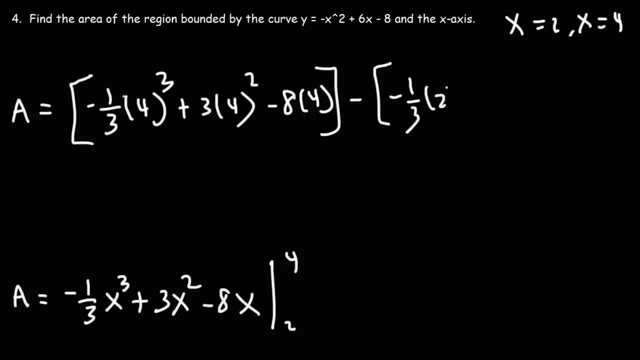 Let's plug in 2.. And now, at this point we just got to do the math. So 4 cubed is 64.. 4 squared is 64.. 16 times 3, that's 48.. 8 times 4 is 32.. 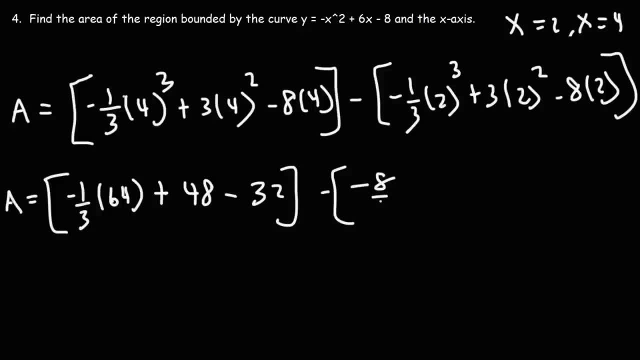 2 to the 3rd is 8.. So this becomes negative 8 over 3.. 2 squared is 4 times 3 is 12.. 8 times 2 is 16.. So right now we have negative 64 over 3.. 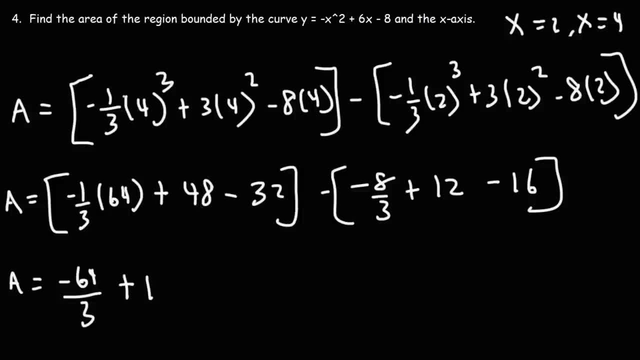 48 minus 32, that's positive 16.. Here we need to distribute the negative sign. So this is going to be positive 8 over 3.. 12 minus 16 is negative 4 times the negative 1 out in front here. 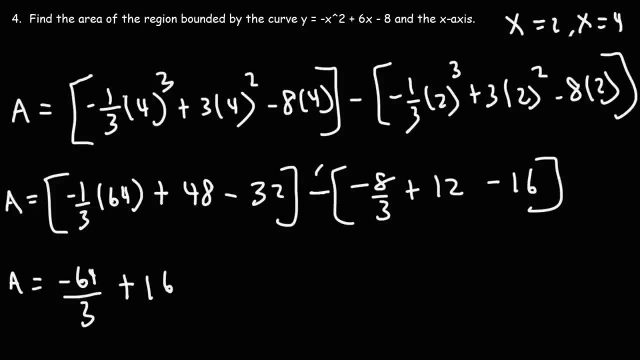 here we need to distribute the negative sign, so this is going to be positive 8 over 3.. 12 minus 16 is negative 4 times the negative 1 out in front here. that's going to be positive 4.. Now we can combine these two, since they're like terms. 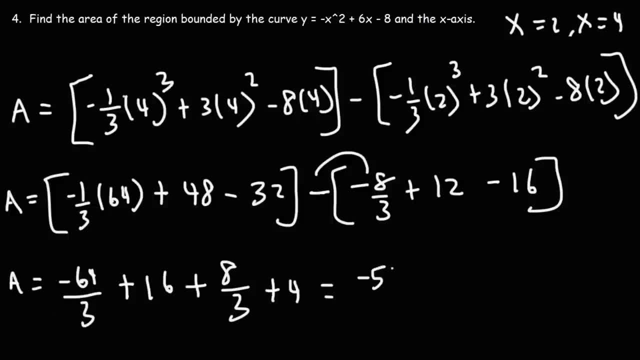 Negative 64 plus 8 is negative 56. And then 16 plus 4 is 20.. I'm going to write that as 20 over 1.. And then to get common denominators, I'm going to multiply the top and bottom by 3.. 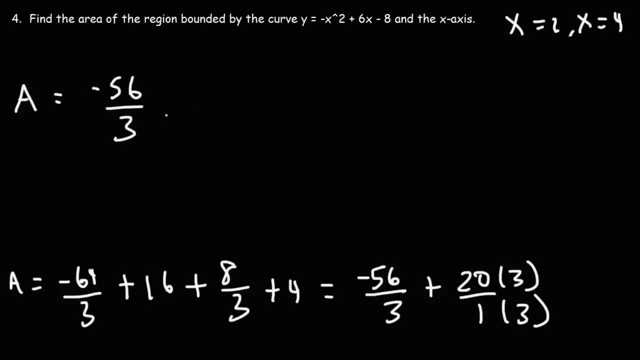 So a equals negative 56 over 3, and then 20 times 3 is 60.. Negative 56 plus 60 is 4.. So the total area of the shaded region is 4 over 3 square units. Now let's work on one more problem. 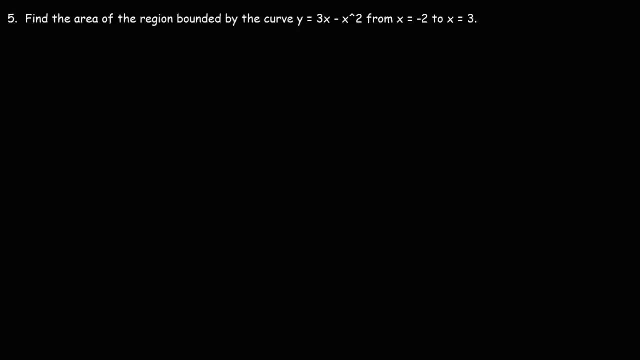 Find the area of the region bounded by the curve. Y equals 3x minus x. squared from x equals negative 2 to x equals 3.. Well, let's begin by drawing a graph And let's find the x-intercepts. So let's replace y with 0.. 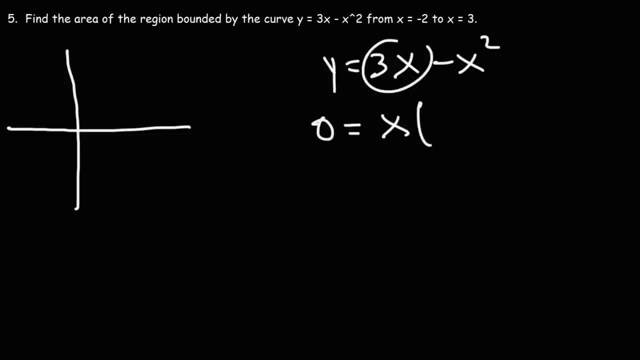 For this one, I'm going to factor out an x. 3x divided by x is 3.. 3x divided by x is 3.. Negative x squared divided by x is negative x. Now, if we set each factor equal to 0, we get x equals 0.. 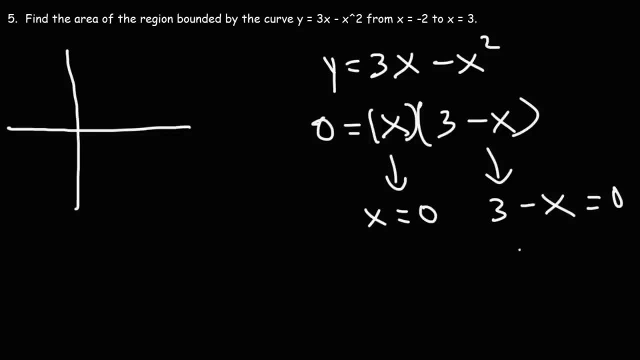 And here we get 3 minus x is 0. Add in x to both sides, we get x equals 3.. So we have an intercept: at x equals 0 and at x equals 3. Which means and we have a negative in front of the x squared. so we know the parabola. 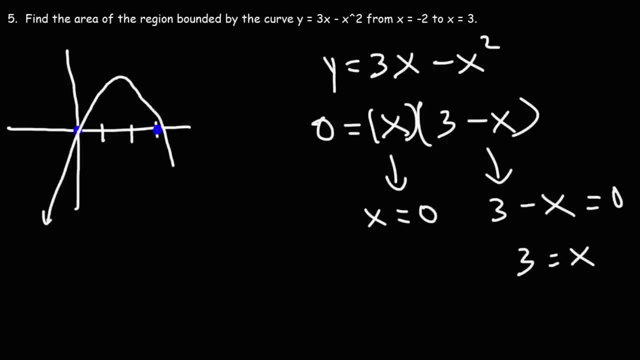 It opens downward, Kind of like this. Now I'm going to have to extend this side a little bit longer. The reason for that is we want to integrate it, or find the area from negative 2 to positive 3.. So we're going to need this part of the graph. 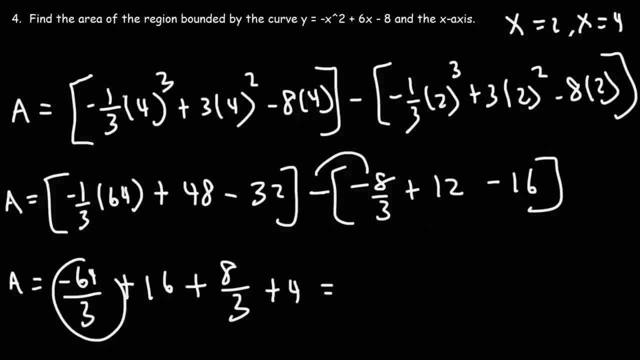 That's going to be positive 4.. Now we can combine these two, since they're like terms: Negative: 64 plus 8 is negative 56. And then 16 plus 4 is 20.. I'm going to write that as 20 over 1.. 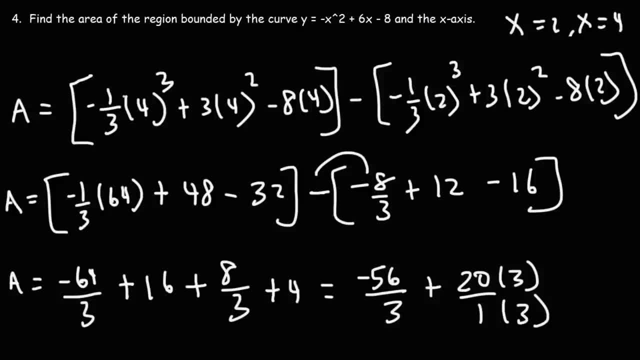 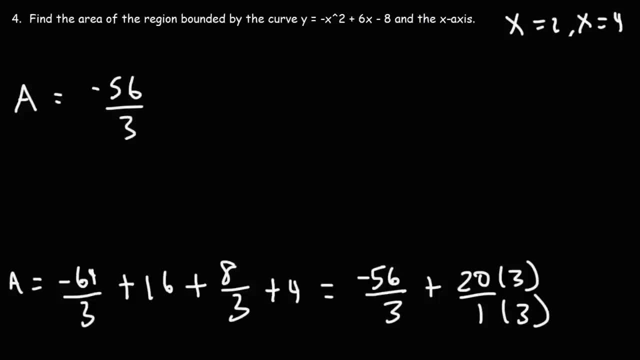 And then to get common denominators, I'm going to multiply the top and bottom by 3.. So 8 equals negative 56 over 3. And then 20 times 3 is 60.. Negative 56 plus 60 is 4.. 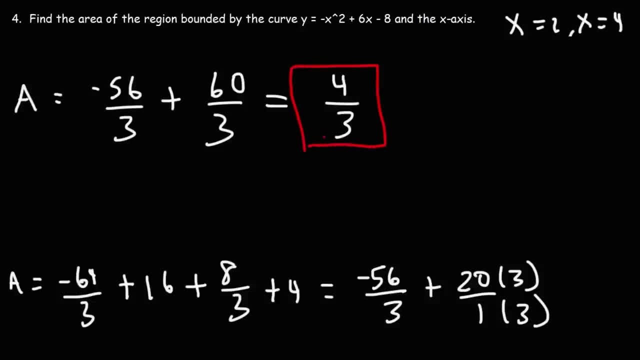 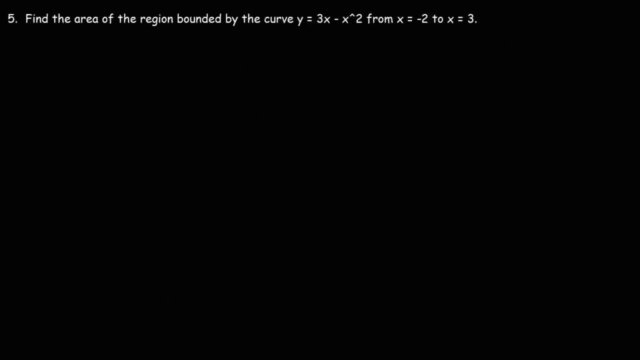 So the total area of the shaded region is 4 over 3 square units. Now let's work on one more problem. Find the area of the region bounded by the curve y equal 3x minus x, squared from x equal negative 2 to x equal 3.. 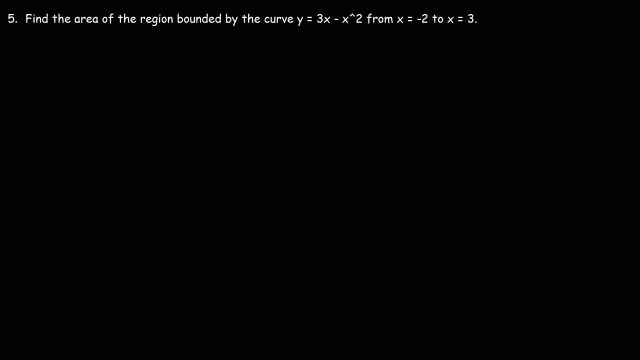 three. Well, let's begin by drawing a graph And let's find the x-intercepts. So let's replace y with zero For this one. I'm going to factor out: an x 3x divided by x is 3.. 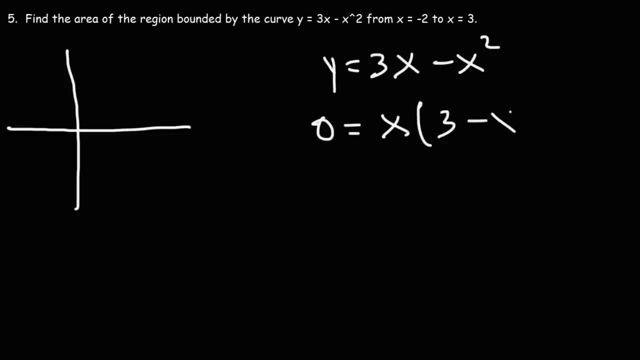 3 negative x squared divided by x is negative x. Now, if we set each factor equal to zero, we get x equals zero. And here we get 3 minus x is zero. Add in x to both sides, we get x equals 3.. So we have an intercept: at x equals zero and at x equals 3. Which means and we: 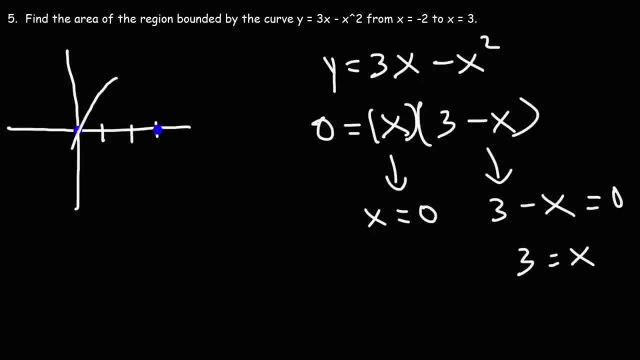 have a negative in front of the x squared. so we know the parabola: It opens downward, Kind of like this. Now I'm going to have to extend this side a little bit longer. The reason for that is we want to integrate it, or find the area from negative 2 to positive 3.. 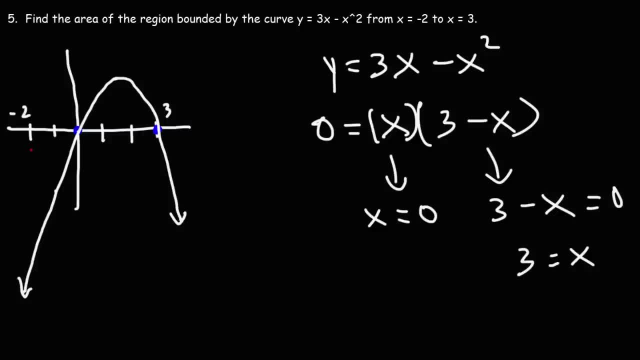 So we're going to need this part of the graph as well as this part. So here we have a positive area and here we have a negative area. But we can't use symmetry and just take one side and multiply it by 2. We have to break this into two separate integrals. 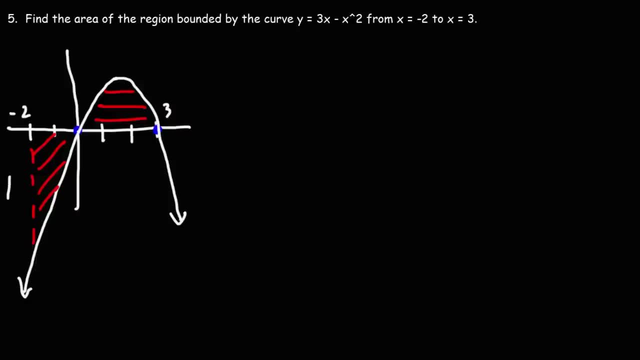 So let's call this area 1 and we'll call this area 2.. The total area is going to be the absolute value of area 2 plus area 1.. Now area 2 is positive. So once we remove the absolute value, 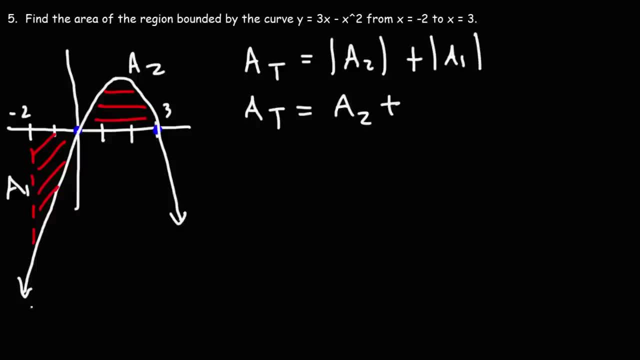 symbol, it's just A2.. A1 is a negative value, So in order to keep it positive, we need to add a negative sign to it. So the total positive area is going to be the absolute value of area 2.. It's going to be A2 minus A1 in this example. 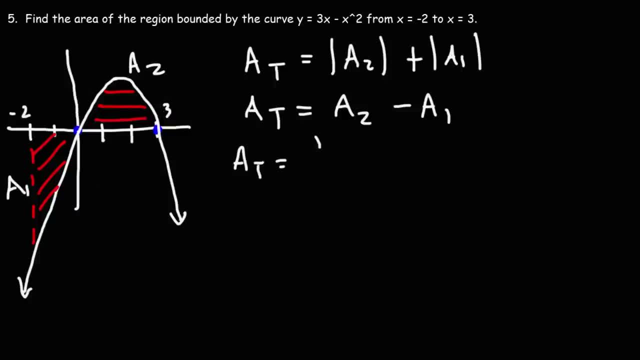 Now this area is simply the definite integral, from 0 to 3, of the function 3x minus x squared. Now for the other one, we have negative. We need to integrate it from negative 2 to 0. But we're dealing with the same function: 3x minus x squared. 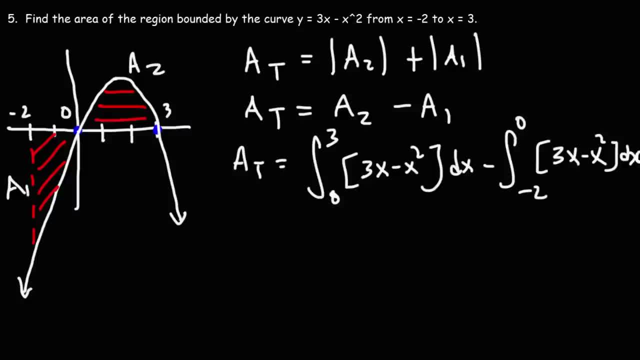 So now that we have this expression, all we got to do is just do the work. So the antiderivative of 3x is going to be 3x squared over 2.. And for x squared, it's just x cubed over 3.. And here it's going to be evaluated from 0 to 3.. 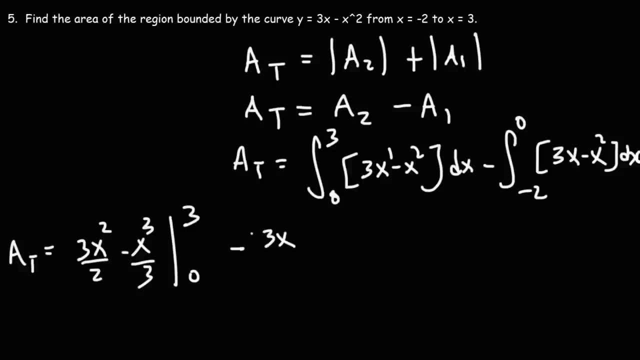 And then for the second part, we'll have the same expression, But we need to keep in mind that there's a negative sign in front of it. But this time we're going to evaluate it from negative 2 to 0. So, substituting 3 into this expression, we have 3 times 3 squared over 2 minus. 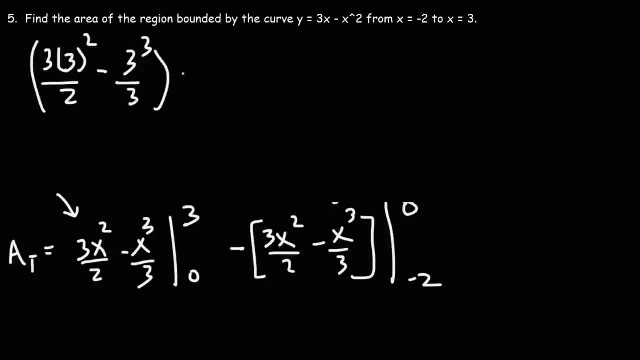 3 to the third over 3.. And then, when we plug in 0, this entire thing will be 0.. So this is just area 2.. Now for this part. once we plug in 0, everything is 0.. 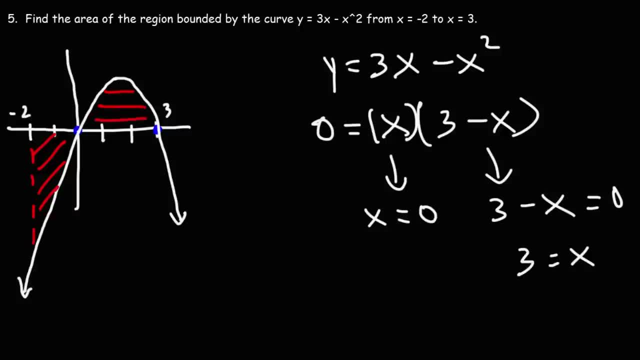 As well as this part. So here we have a positive area and here we have a negative area. But we can't use symmetry and just take one side and multiply it by 2. We have to break this into two separate integrals. So let's call this area 1 and we'll call this area 2.. 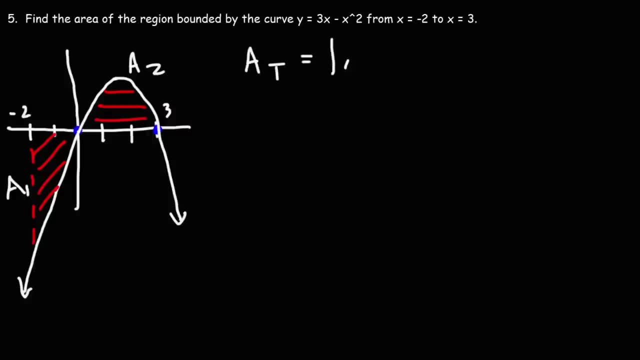 The total area is going to be the absolute value of area 2 plus area 1.. Now area 2 is positive, so once we remove the absolute value symbol, it's just a2.. a1 is a negative value, so in order to keep it positive, we need to add a negative sign to it. 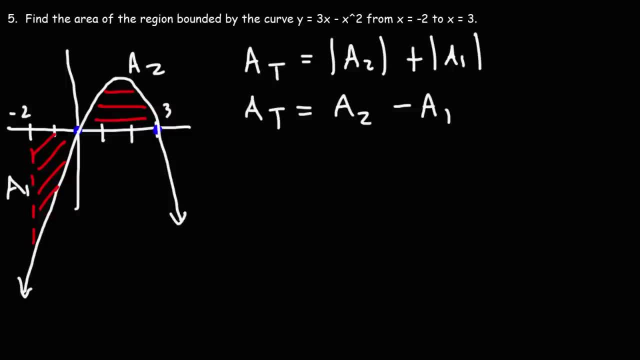 So the total positive area It's going to be a2 minus a1 in this example. Now this area is simply the definite integral from 0 to 3 of the function 3x minus x squared. Now for the other one we have negative. 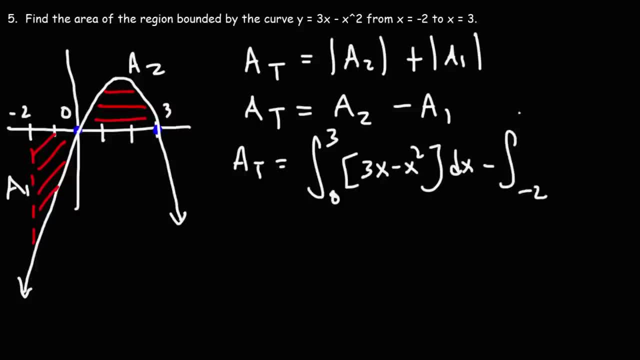 We need to integrate it from negative 2 to 0.. But we're dealing with the same function: 3x minus x squared. So now that we have this expression, all we've got to do is just do the work. So the antiderivative of 3x is going to be 3x squared over 2.. 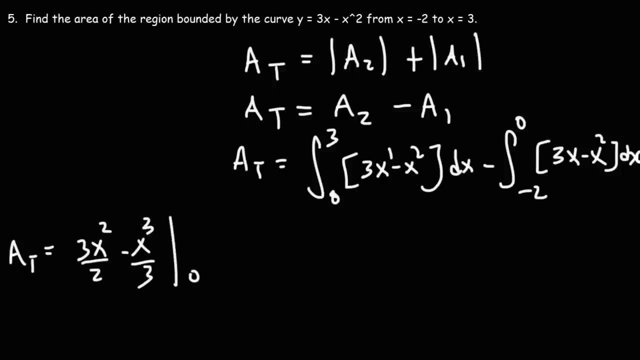 And for x squared, it's just x cubed over 3.. And here it's going to be evaluated from 0 to 3.. And then for the second part, we'll have the same expression, But we need to keep in mind that there's a negative sign in front of it. 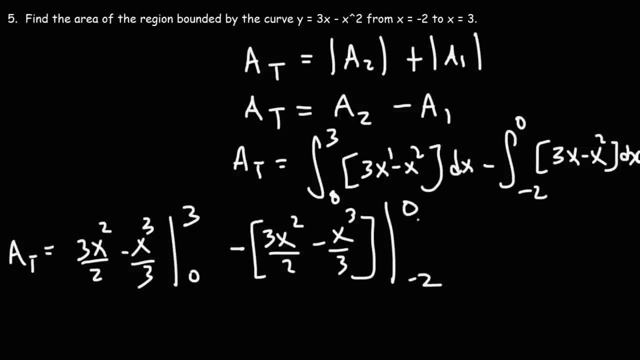 But this time we're going to evaluate it from negative 2 to 0. So substituting 3 into this expression, we have 3 times 3 squared over 2, minus 3 to the third over 3.. And then when we plug in 0, this entire thing will be 0.. 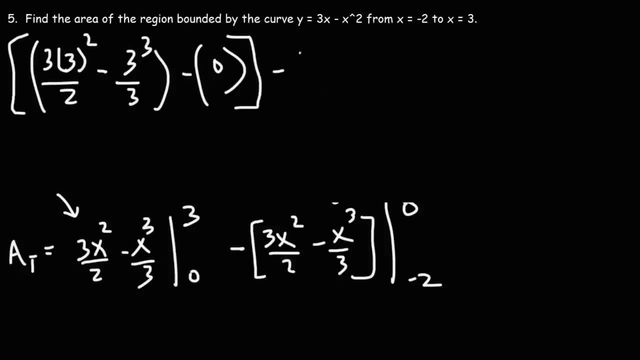 So this is just area 2.. Now for this part. once we plug in 0,, everything is 0. And then, minus, we need to plug in negative 2. So it's going to be 3 times negative 2 squared over 2 minus negative 2.. 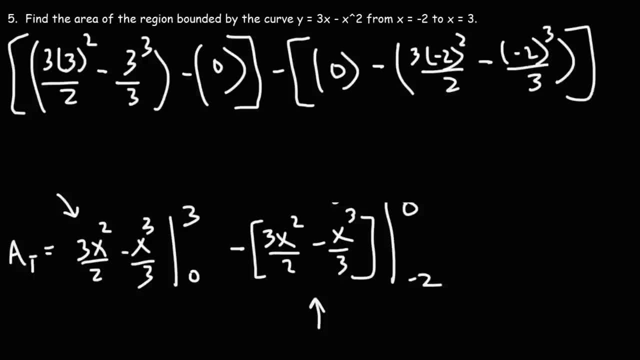 2 to the third over 3.. 3 squared is 9 times 3,, that's 27.. So this is 27 over 2.. Here, 3 to the third is 27 divided by 3.. So this is going to be 9.. 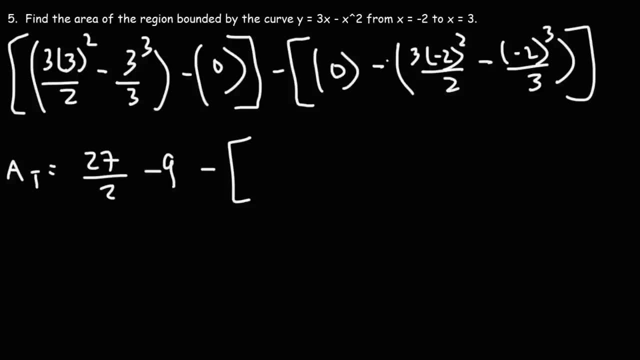 And then minus. And then we have another negative sign here, The 0, we could just not worry about Negative 2 squared is 4, divided by 2 is 2 times 3.. That's going to be 6.. Here we have negative 2 to the third. 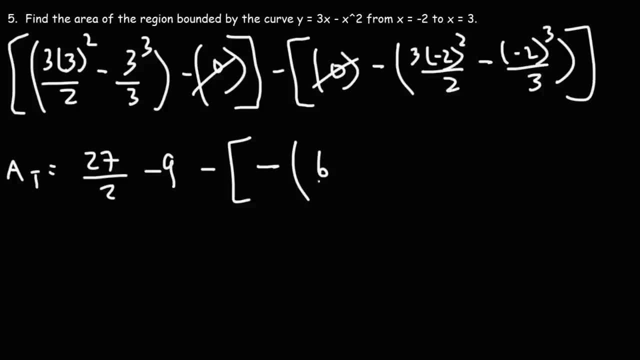 That's negative 8 times a negative 1. That's positive 8.. So plus 8 over 3.. All right, These two negative signs will cancel. So that's just going to be 0.. That's going to be positive. 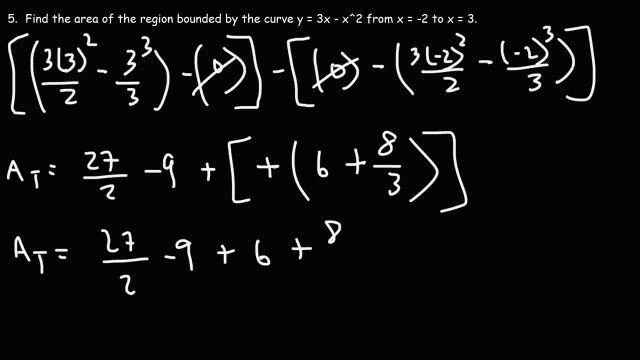 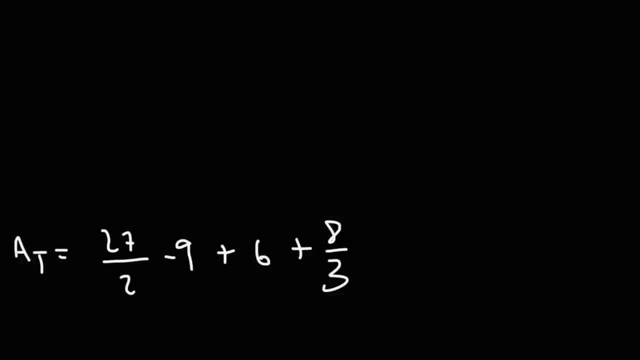 So we can just write it out like this: Plus 6 plus 8 over 3.. Negative 9 plus 6, that's going to be negative 3.. Now what we need to do at this point is we need to get common denominators. 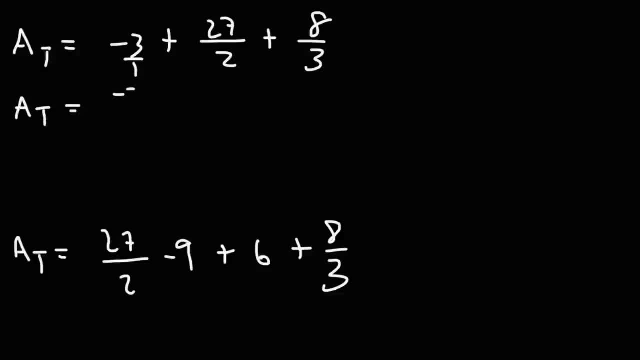 So let's try to get a common denominator of 6.. So negative: 3 over 1, I'm going to multiply it by 6 over 6.. 27 over 2, I'm going to multiply it by 3 over 3.. 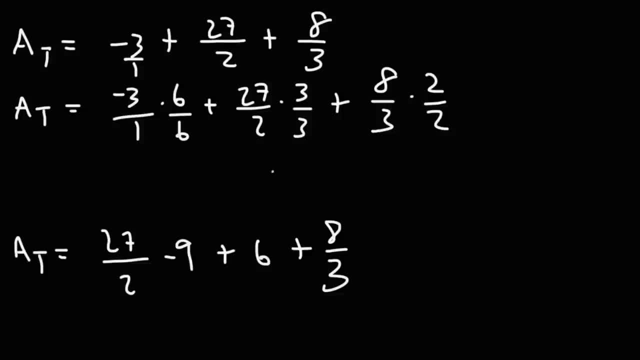 And 8 over 3, I'm going to multiply it by 2 over 2.. So this is negative 18 over 6.. 27 times 3.. 20 times 3 is 60.. 7 times 3 is 21.. 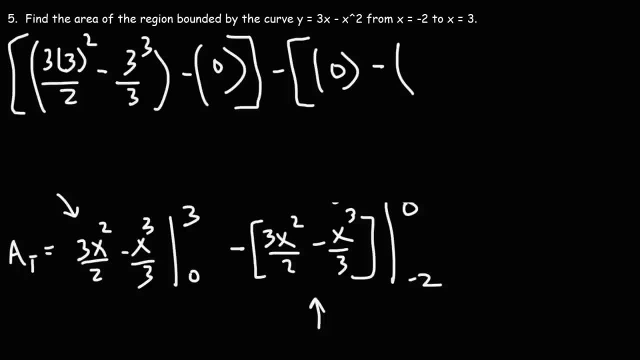 And then minus, we need to plug in negative 2.. So it's going to be 3 times negative 2 squared over 2 minus minus 2 squared over 2 minus negative 2 squared over 2 minus negative 2.. negative 2 to the 3rd over 3.. 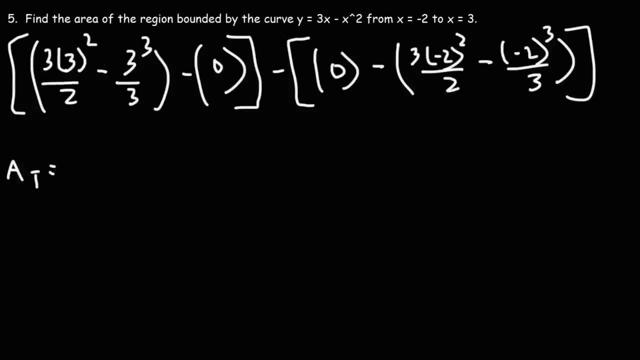 3 squared is 9, times 3,, that's 27,. so this is 27 over 2.. Here, 3 to the 3rd is 27 divided by 3, so this is going to be 9.. 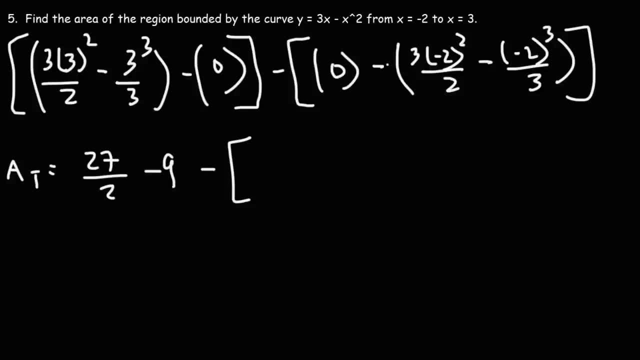 And then minus. and then we have another negative sign here, The 0. we could just not worry about. Negative: 2 squared is 4, divided by 2 is 2, times 3, that's going to be 6.. 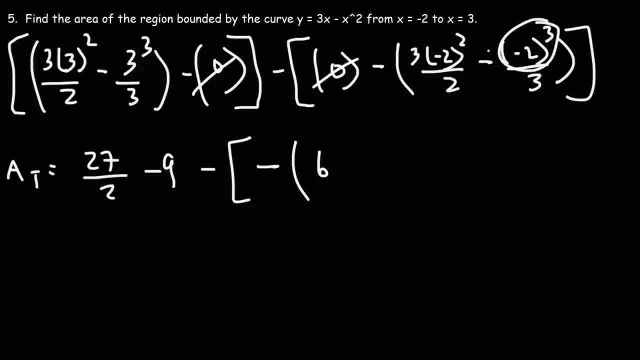 Here we have negative 2 to the 3rd, that's negative 8, times a negative 1, that's positive 8. So plus 8 over 3.. Alright, these two negative signs, These two positive signs will cancel. so that's just going to be positive. 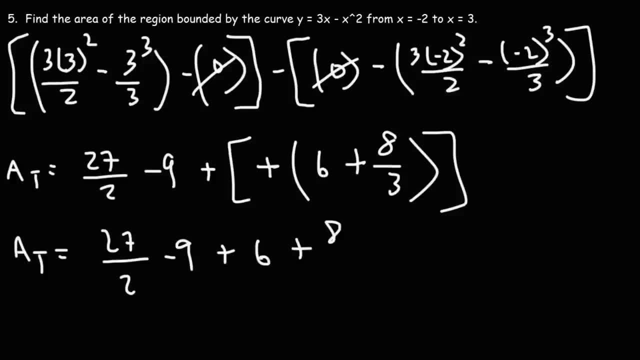 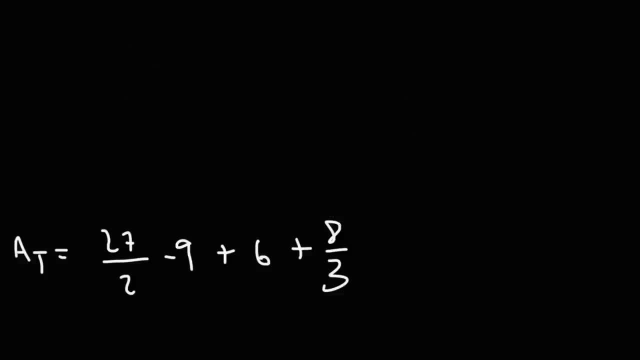 So we can just write it out like this: plus 6, plus 8 over 3.. Negative 9 plus 6,, that's going to be negative 3.. Negative 9 plus 6,, that's going to be negative 3.. 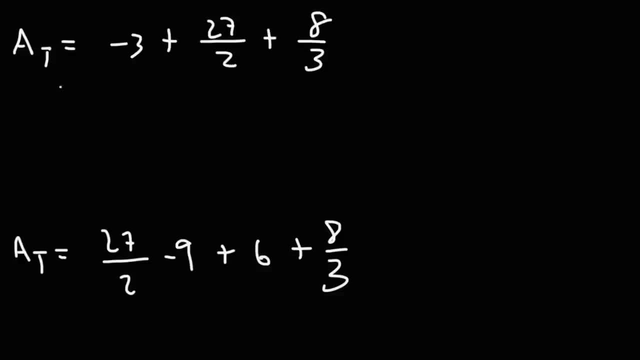 Now what we need to do at this point? Now, what we need to do at this point is we need to get common denominators. So let's try to get a common denominator of 6.. So, negative 3 over 1, I'm going to multiply by 6 over 6.. 27 over 2, I'm going to multiply by 3. 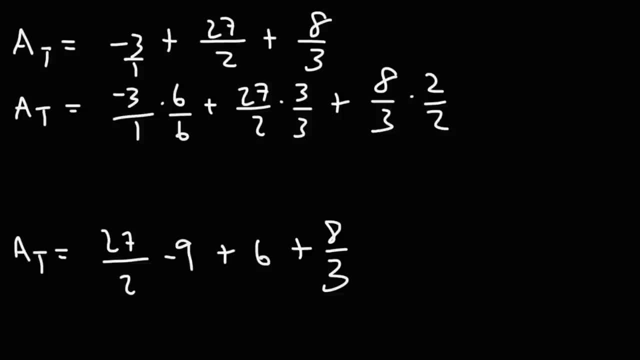 over 3.. And 8 over 3, I'm going to multiply by 2 over 2.. So this is negative: 18 over 6.. 27 times 3.. 20 times 3 is 60.. 7 times 3 is 21.. When you add 60 and 21,, you get 81. 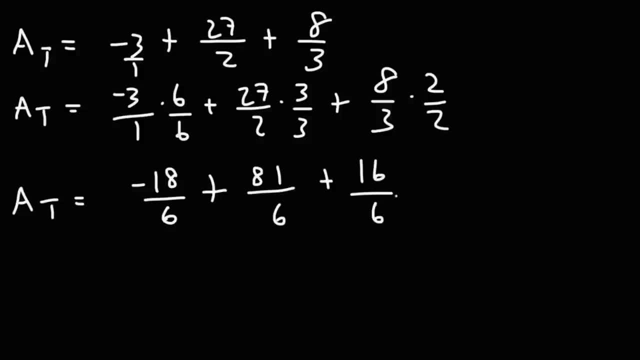 And 8 times 2 is 16.. Negative 18 plus 16, that's going to be negative 2.. So we have 81 over 6 minus 2 over 6. And 81 minus 2 is 79. So we have 79 over 6.. 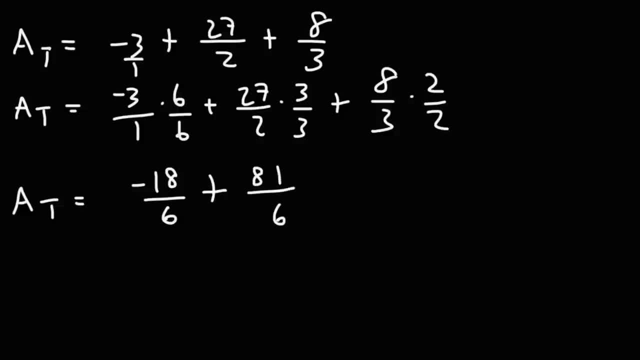 When you add 60 and 21,, you get 81. So this is negative 18 over 6. And 8 times 2 is 16.. Negative 18 plus 16, that's going to be negative 2. So we have 81 over 6 minus 2 over 6.. 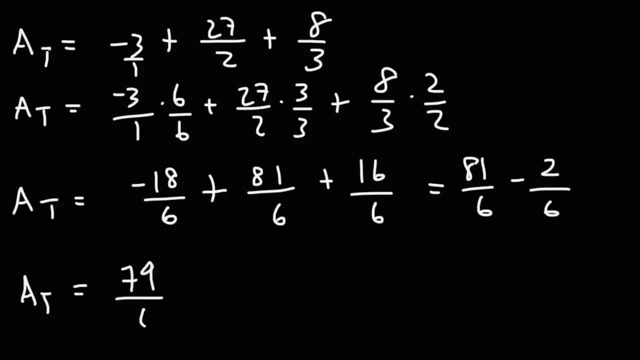 And 81 minus 2 is 79. So we have 79 over 6. And if we want to, we can break this up so that we can get a mixed fraction. 79 is 60 plus 18. Plus 1.. 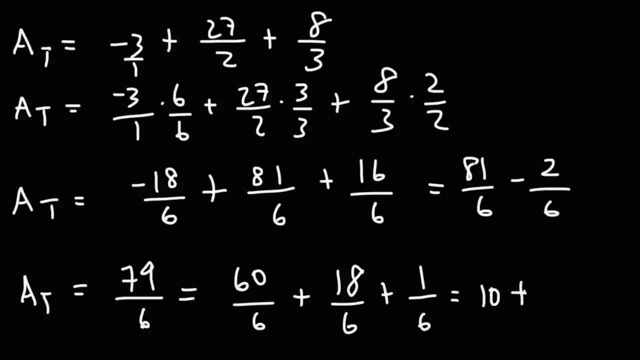 60 divided by 6 is 10.. 18 divided by 6 is 3.. And we have this. So 10 plus 3 is 13.. So we have 13 plus 1 over 6.. Whereas a mixed fraction 13 and 1: 6.. 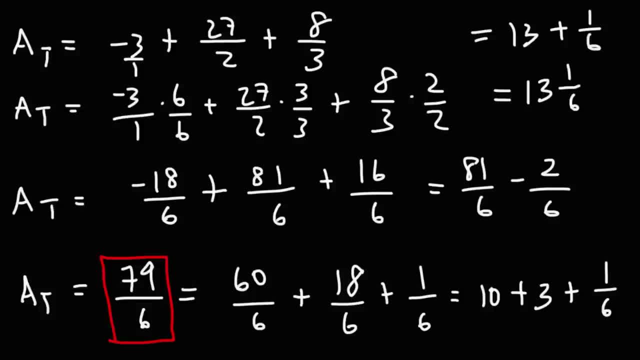 So the total area. we can leave it as an improper fraction: 79 over 6.. Or we can leave it as a mixed number: 13 and 1: 6.. So that's basically it for this video. Now you know how to calculate the area under the curve. 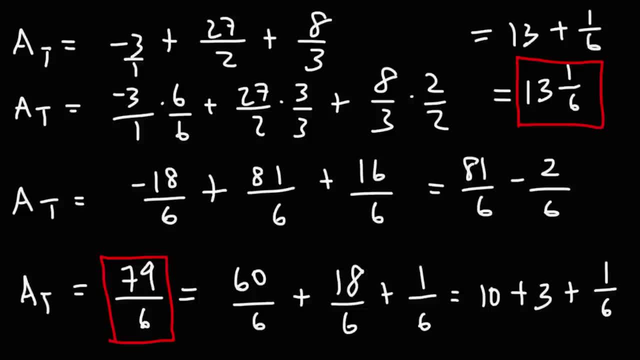 I do have other videos in calculus that is related to this topic, Such as how to calculate the area between curves. Now you can do a YouTube search to find that video Or you can check out the links in the description section below. I also have other videos like the disk method. 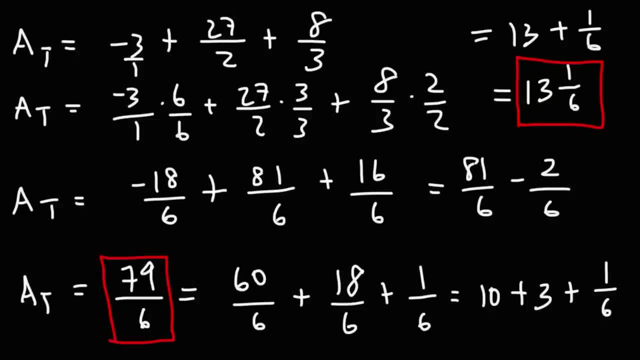 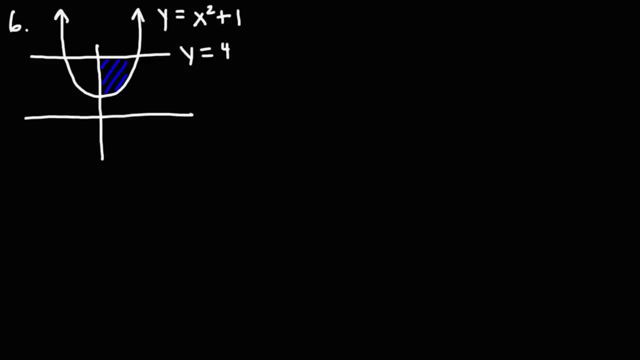 You know how to calculate the volume using the disk method, the shell method And by using cross-selecting. So feel free to take a look at those videos when you get a chance, And thanks for watching. Consider this problem: Find the area of the shaded region bound by the curves y equal x squared plus 1 and y equal 4.. 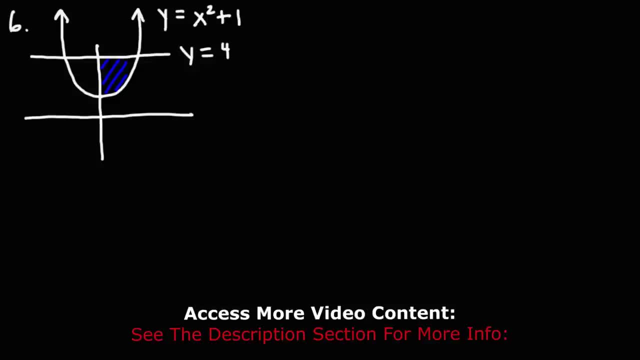 As shown on the screen. Now this one. there's different ways in which we can do this, But let's use this formula. The area is the integral from c to d of g, of y, dy. Now recall that y is f of x. 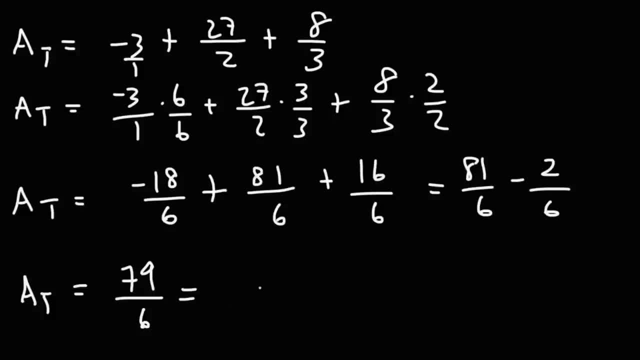 And if we multiply by 6 over 6,, we get 7 over 6.. If we want to, we can break this up so that we can get a mixed fraction: 79 is 60 plus 18 plus 1.. 60 divided by 6 is 10.. 18 divided by 6 is 3. And we have this. 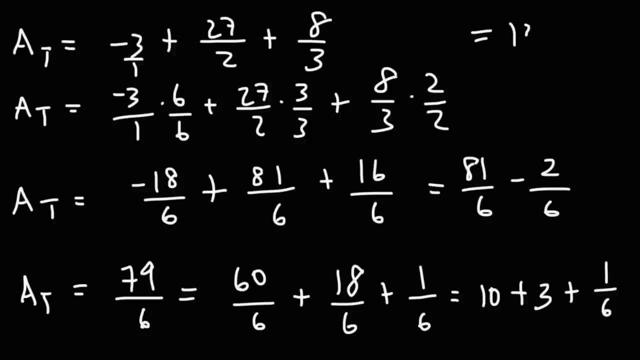 So 10 plus 3 is 13.. So we have 13 plus 1 over 6,, whereas a mixed fraction 13 and 1, 6.. So the total area: we can leave it as an improper fraction 79 over 6, or we can leave it as a mixed number 13 and 1, 6.. 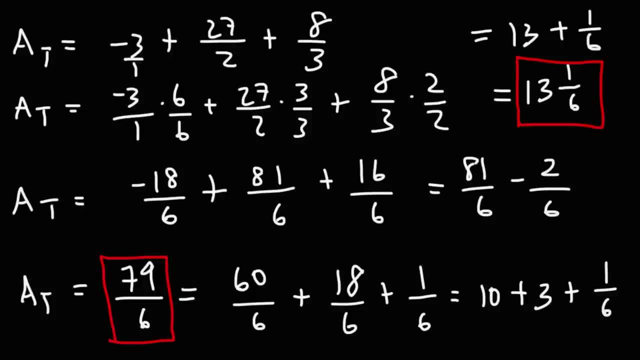 So that's basically it for this video. Now you know how to calculate the area under the curve. I do have other videos in calculus that is related to this topic, such as how to calculate the area between curves. Now you could do a YouTube search. 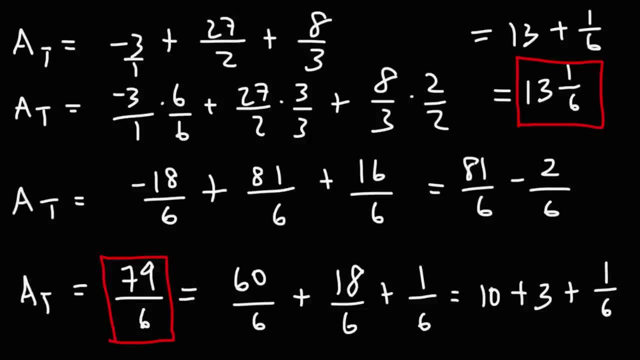 to find that video, or you could check out the links in the description section below. I also have other videos on how to calculate the area under the curve, So feel free to take a look at those videos when you get a chance, and thanks for watching. 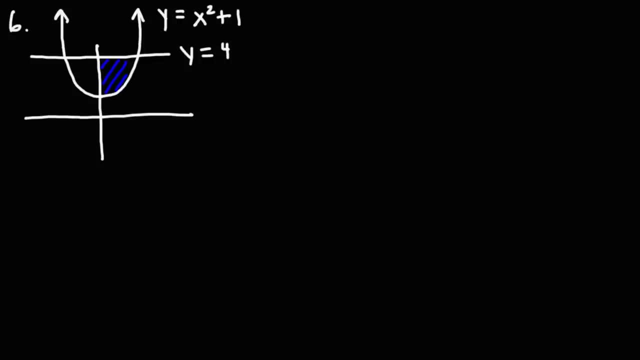 Consider this problem. Find the area of the shaded region bounded by the curves: y equal x squared plus 1, and y equal 4, as shown on the screen. Now this one. there's different ways in which we can do this, But let's use this formula. The area is the integral from c to d, of g, of y, dy. 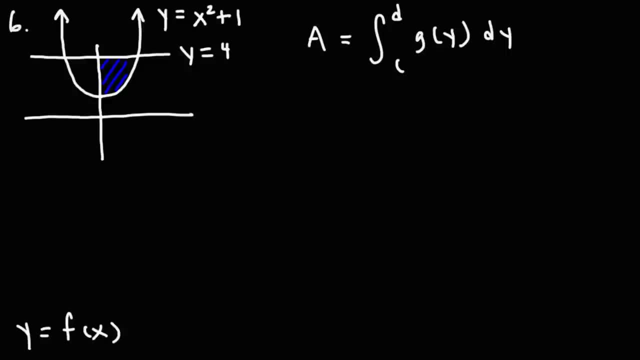 Now recall that y is f of x and x is g of y. So if you're using this formula, what you need to do is you need to solve for y in this equation. I mean not y, but you need to solve for x in that equation. 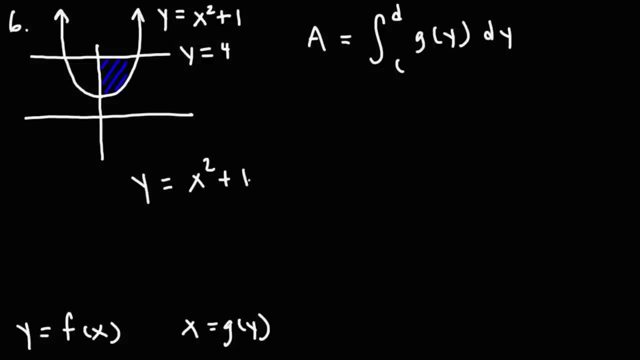 So we have: y is equal to x squared plus 1.. Solving for x, we have: y minus 1 is equal to x squared. So x is going to be the square root of y minus 1.. And since x is g of y, g of y is the square root. 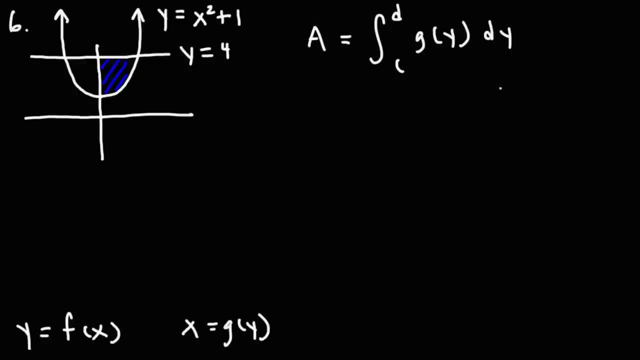 And x is g of y. So if you're using this formula, What you need to do is you need to solve for y in this equation. I mean not y, but you need to solve for x in that equation. So we have: y is equal to x squared plus 1.. 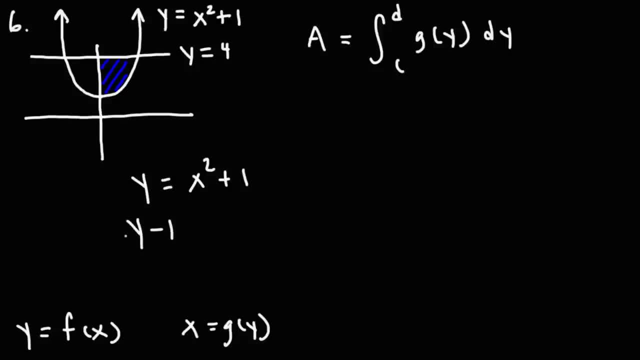 Solving for x, we have: y minus 1 is equal to x squared, So x is going to be the square root of y minus 1.. And since x is g of y, g of y is the square root of y minus 1.. 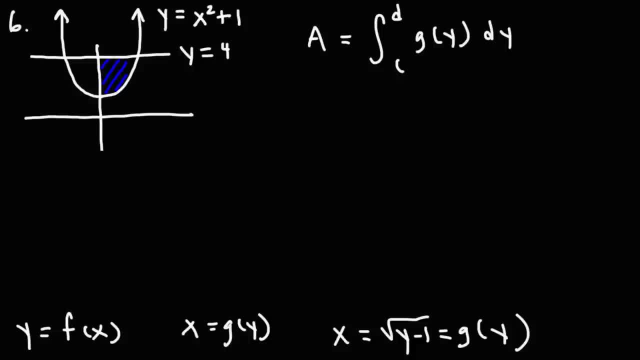 Now the next thing we need to know are our c and d values. This is d and this is c. It's very clear for us to see that d is equal to 4.. c and d are y values. c is 1.. 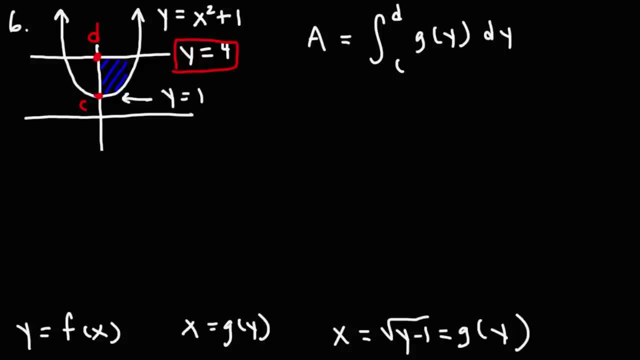 Because when x is 0, y is equal to 1.. Using that formula, So, the area is the integral of 1 to 4.. Of g, of y, which is the square root of y minus 1.. Which we can write it like this: 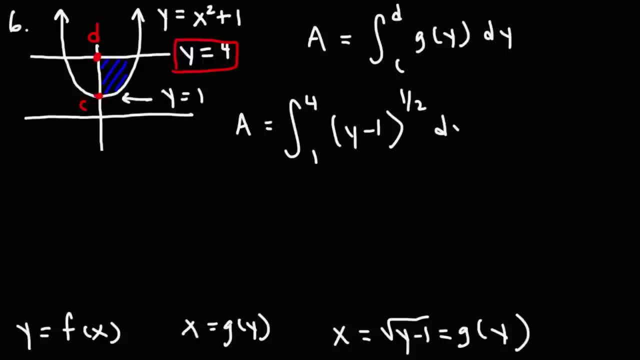 It's y minus 1 raised to the 1 half d y. So let's go ahead and find the antiderivative of that expression. So we're going to add 1 to 1 half, Which is 3 over 2.. 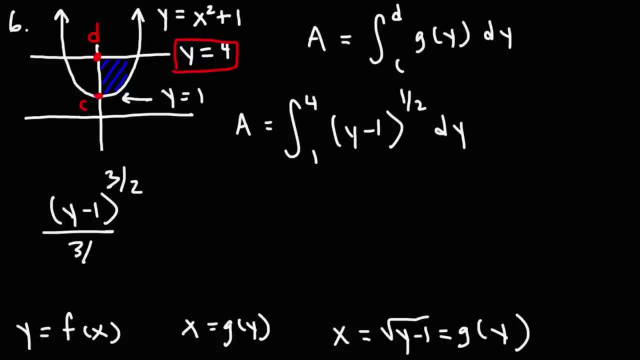 And then we're going to divide by 3 over 2. Which is the same as multiplying it by 2 over 3.. The derivative of y minus 1 is just 1.. So we don't need to worry about that. If you were to use u substitution, you would still get this answer. 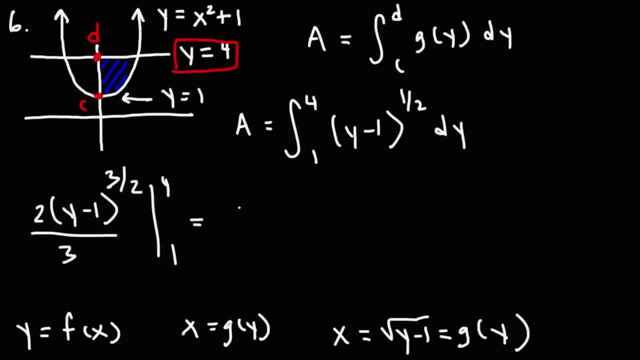 Now let's evaluate it from 1 to 4.. So this is 2 raised to the y minus 1.. Well, this is 2 times 4 minus 1 raised to the 3 over 2 over 3. And then minus. 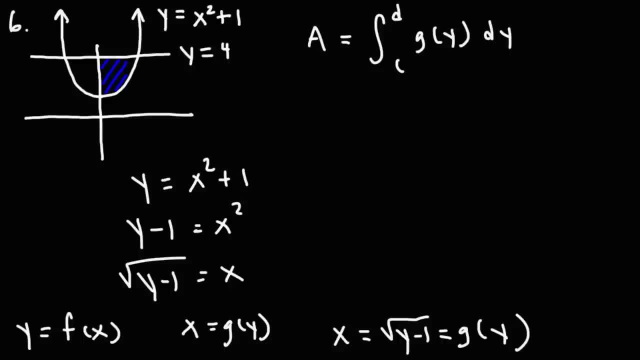 of y minus 1.. Now the next thing we need to know are our c and d values. This is d and this is c. It's very clear for us to see that d is equal to 4.. c and d are y values. c is 1, because when x is 0,, y is equal to 1.. 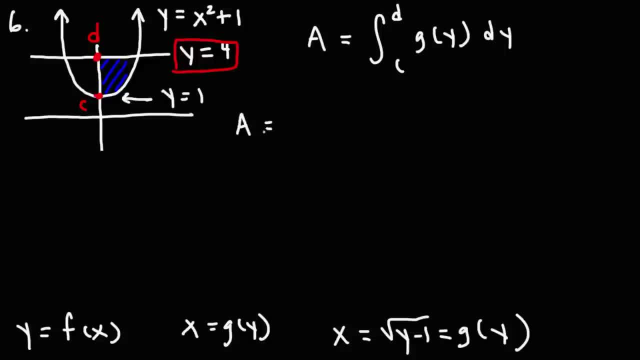 Using that formula. So the area is the integral of 1 to 4 of g, of y, which is the square root of y minus 1, which we can write it like this: It's y minus 1 raised to the 1 half dy. So let's go ahead and find the antiderivative. 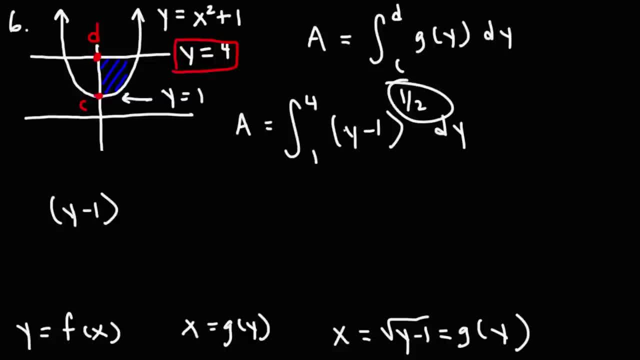 of that expression. So we're going to add 1 to 1 half, which is 3 over 2.. And then we're going to divide by 3 over 2, which is the same as multiplying it by 2 over 3.. The derivative of y minus 1 is just 1.. So we don't need to. 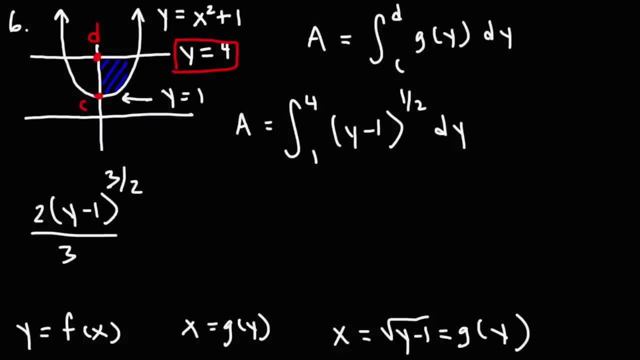 worry about that. If you were to use u substitution, you would still get this answer. Now let's evaluate it from 1 to 4.. So this is 2 raised to the y minus 1, which is well, this is 2 times 4 minus 1 raised to the 3 over 2 over 3,. 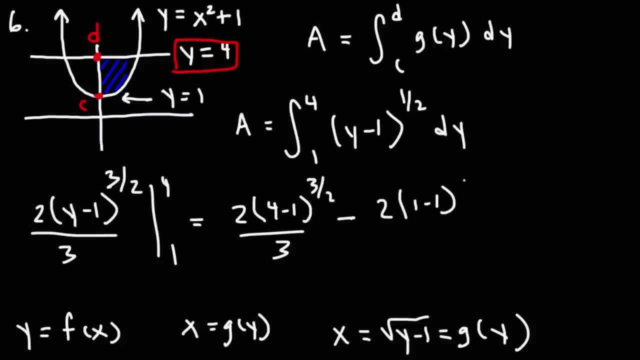 and then minus 2 times 1 minus 1 over 3.. So 4 minus 1 is 3.. 1 minus 1 is just 0. So right now we have 2 over 3.. 3 to the 3 halves, that's 3 to the 3rd. 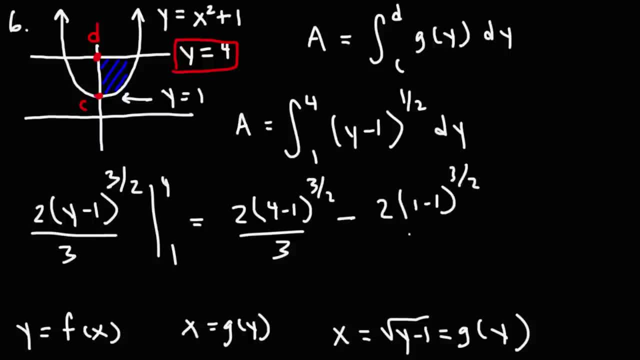 2 times 1 minus 1 over 3.. So 4 minus 1 is 3.. 1 minus 1 is just 0.. So right now we have 2 over 3.. 3 to the 3 halves. 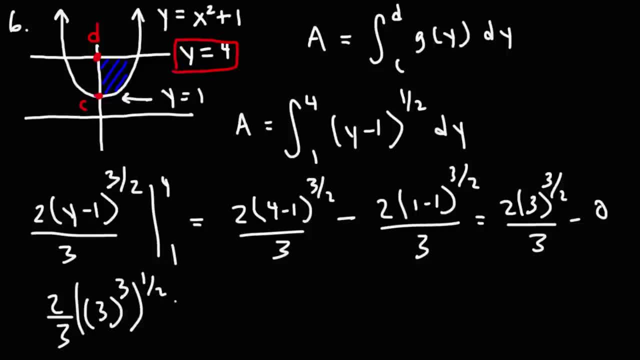 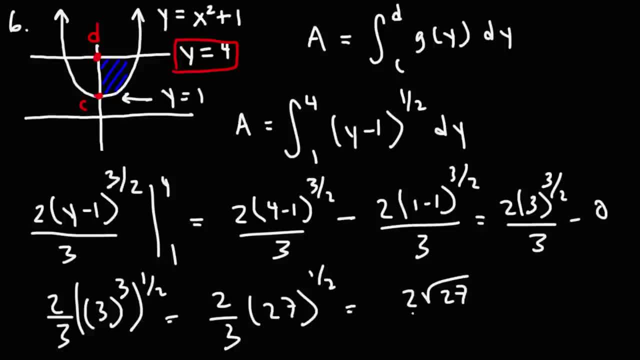 So this is 2 square root, 27 over 3.. Now the square root of 27,. we could simplify that as the square root of 9 times the square root of 3.. The square root of 9 is 3. And so we could cancel that. 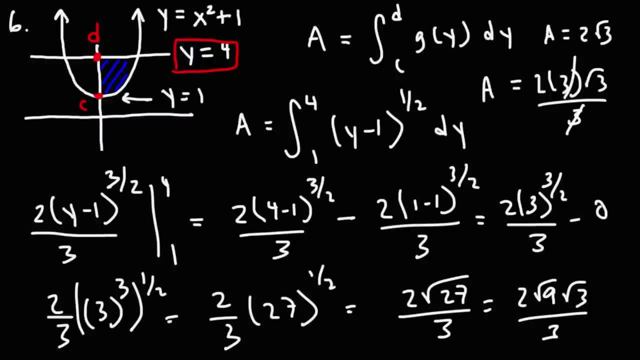 So we get that the area is 2 square root 3.. So that is the area of the shader region for this problem. So that's how you can get the answer in terms of y. Now the other method involves finding the area between two curves. 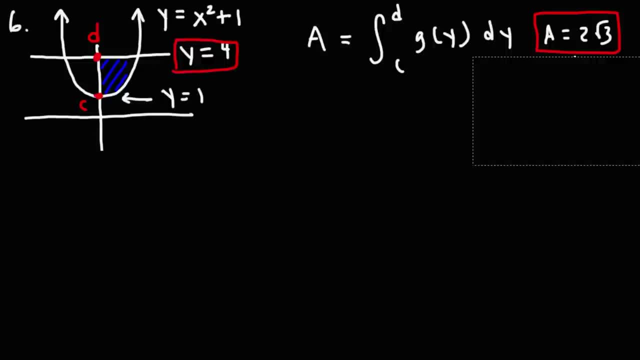 And we can do it in terms of x. So let's say we have two functions. Let's say the top function is f of x, The bottom function is g of x And we want to find the area of the shaded region between those two functions. 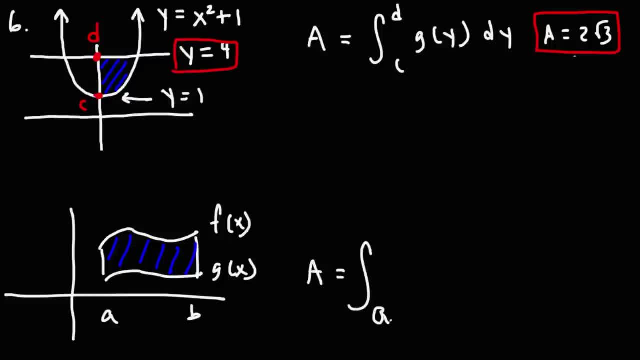 In this case, the area is going to be the difference, It's the definite integral from a to b And it's the difference of the top function f minus the bottom function g. So if we're going to apply this formula to this problem, 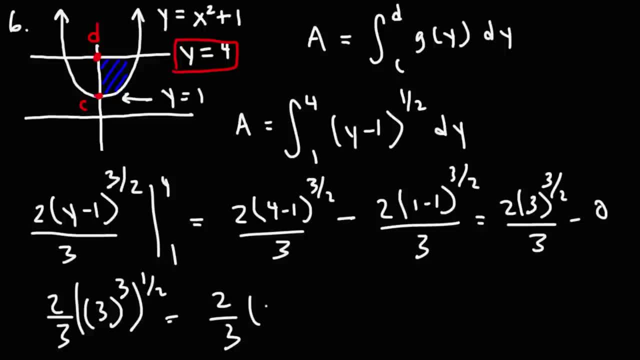 raised to the 1 half, 3 to the 3rd, is 27.. So this is 2 square root 27 over 3.. Now the square root of 27,. we could simplify that as the square root of 9 times the square root of 3.. 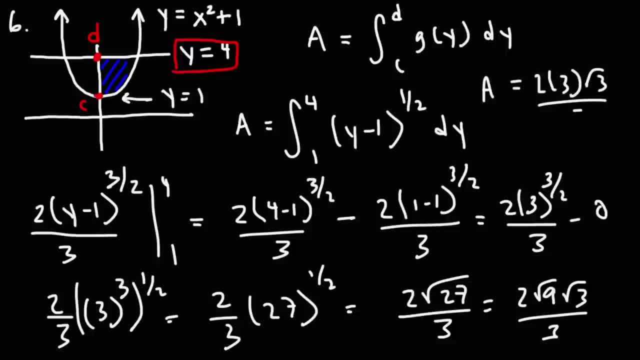 The square root of 9 times the square root of 3 is 27.. So this is 2 square root 27 over 3.. The square root of 9 is 3. And so we could cancel that. So we get that the area is 2 square root 3.. 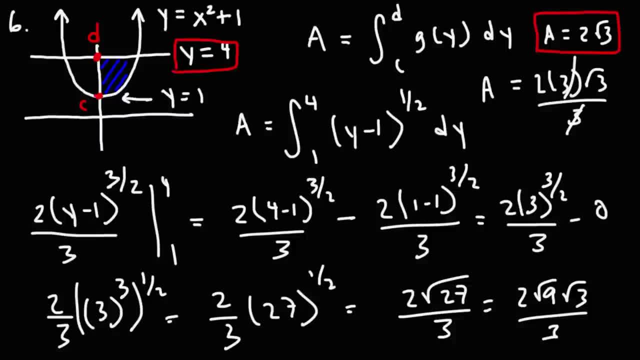 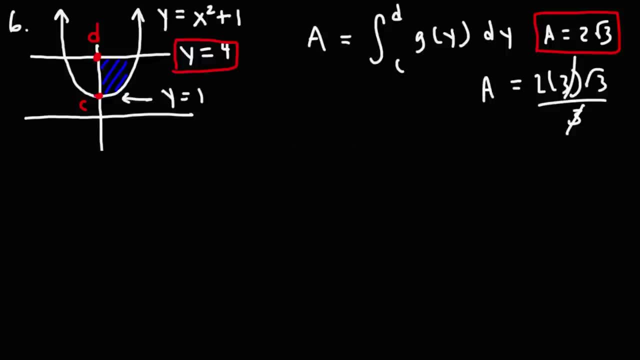 So that is the area of the shader region for this problem. So that's how you can get the answer in terms of y. Now the other method involves finding the area between two curves, And we can do it in terms of x. So let's say we have two functions. 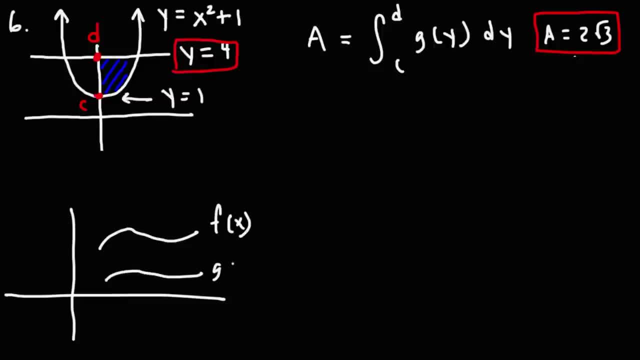 Let's say the top function is f of x, The bottom function is g of x And we want to find the area of the shader region between those two functions. In this case the area is going to be the difference, It's the definite integral from a to b. 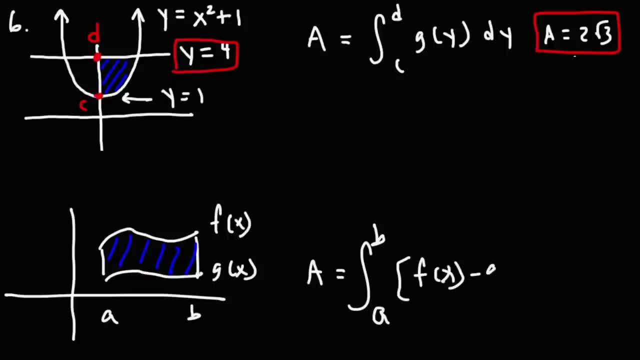 And it's the difference of the area between those two functions. It's the difference of the top function, f, minus the bottom function, g. So if we're going to apply this formula to this problem, instead of using c and d values, we're going to be using a and b values. 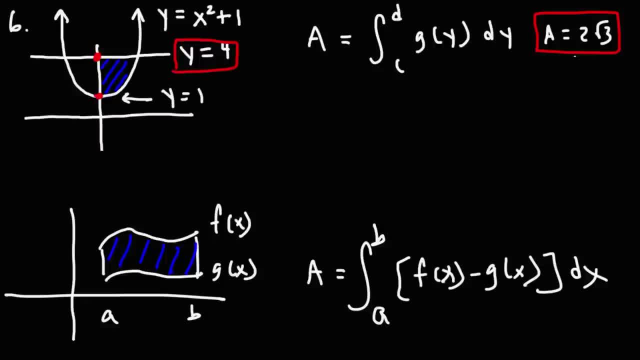 Since it's going to be in terms of x instead of y. So in this case, this is going to be a and this is going to be b. So a is x equals 0.. b is wherever this curve intersects the line. y equals 4.. 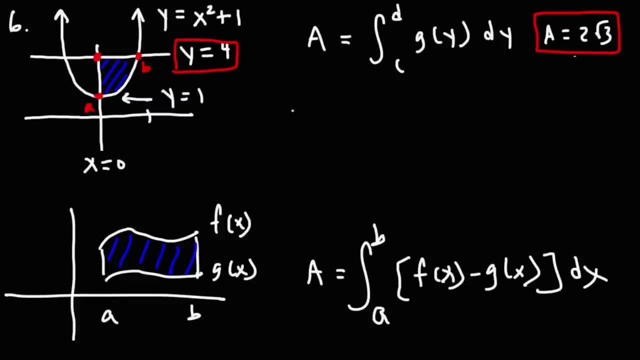 So we have to solve for that. In order to find b, we need to set these two equal to each other And we need to solve for x. So 4 is going to equal x squared plus 1.. Subtracting both sides by 1, we get: 3 is equal to x squared. 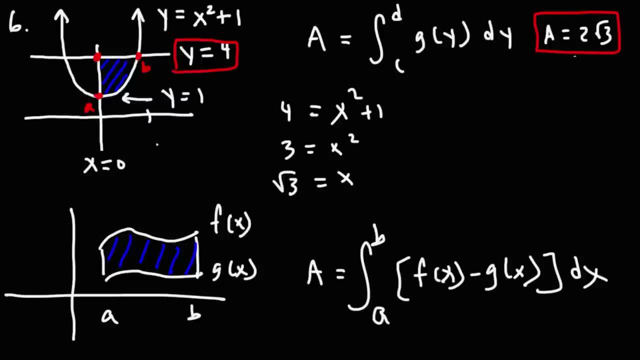 So x is going to be the square root of 3.. So b is positive root 3.. And this part here is negative root 3.. But we don't need that Now. in this example the top function is the line y equals 4.. 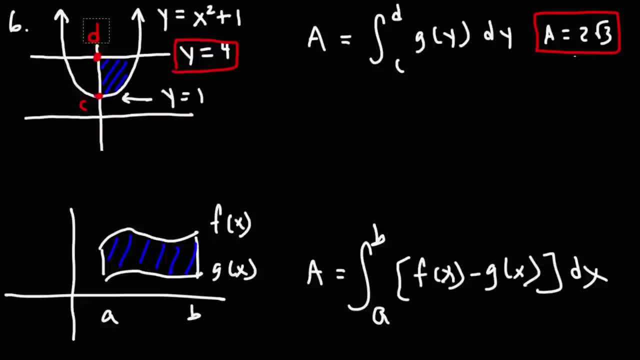 instead of using c and d values, we're going to be using a and b values, Since it's going to be in terms of x instead of y. So in this case, this is going to be a and this is going to be b. 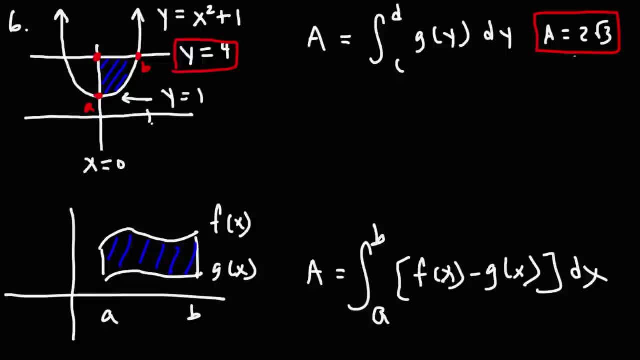 So a is x equals 0.. b is wherever this curve intersects the line y equals 4.. So we have to solve for that. In order to find b, we need to set these two equal to each other And we need to solve for x. 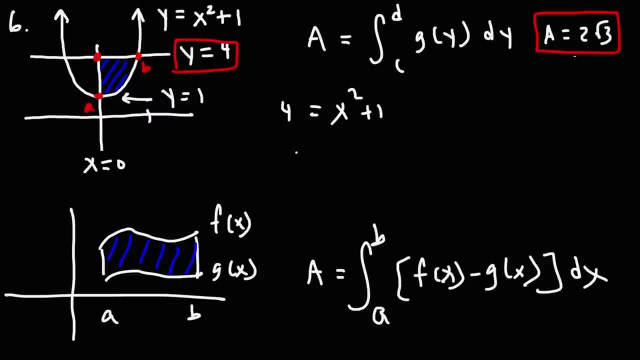 So 4 is going to equal x squared plus 1.. Subtracting both sides by 1, we get 3 is equal to x squared, So x is going to be the square root of 3.. So b is positive root 3.. 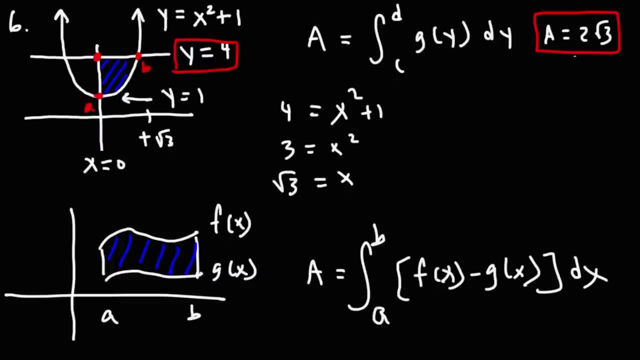 And this part here is negative, root 3.. But we don't need that Now. in this example, the top function is the line y equals 4.. So that's going to be f of x. The bottom function is the curve x squared plus 1.. 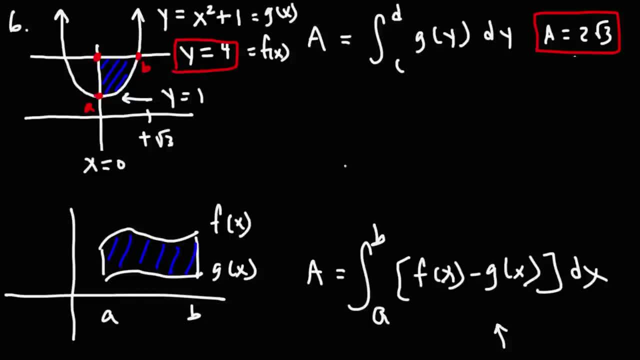 So that's our g of x. So, using this formula, we have this set up. The area is going to be the integral from a to b. a is 0.. b is the square root of 3.. And then f is 4.. 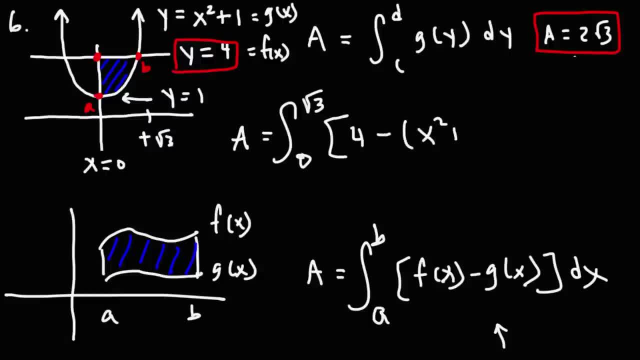 My g of x is 0.. minus g, which is x squared plus 1.. So we could simplify this expression: 4 minus 1 is 3.. So this simplifies to 3 minus x squared if we distribute the negative sign. 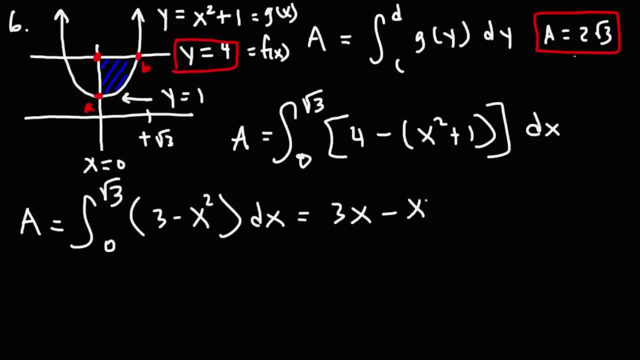 Anti-derivative of 3 is 3x For x squared. it's going to be x cubed over 3, evaluated from 0 to root 3.. So, plugging in root 3, we have 3 times root 3. 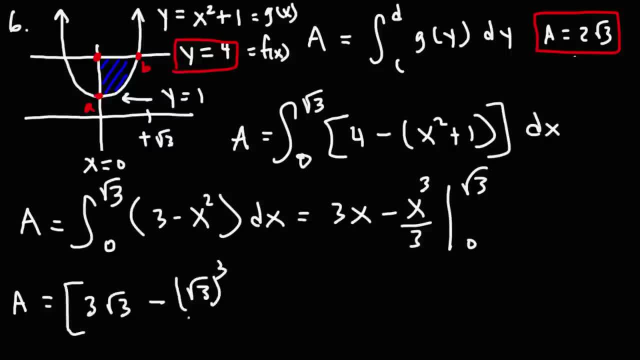 minus root 3 to the third power over 3.. And all of that minus 0.. So root 3 to the third power. So basically we have it 3 times If we multiply the square root of 3 times the square root of 3,. 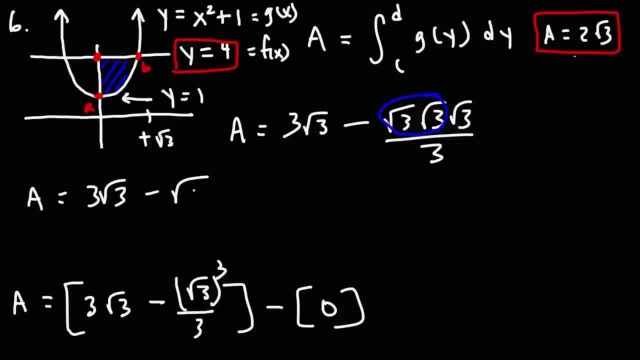 we're going to get the square root of 9.. And the square root of 9 is 3.. So we have this, And 3 divided by 3 is 1.. So we have 3 square root 3 minus 1 square root, 3.. 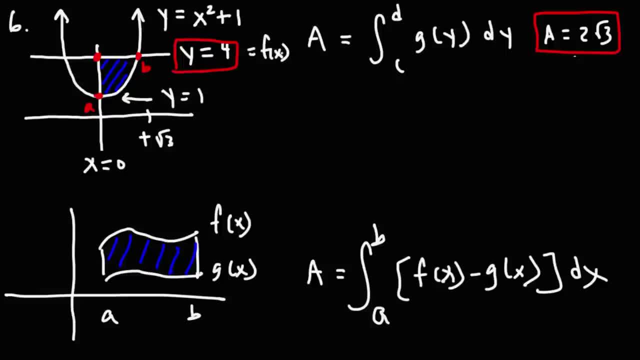 So that's going to be f of x. The bottom function is the curve x squared plus 1.. So that's our g of x. So using this formula, we have this set up. The area is going to be the integral from a to b. 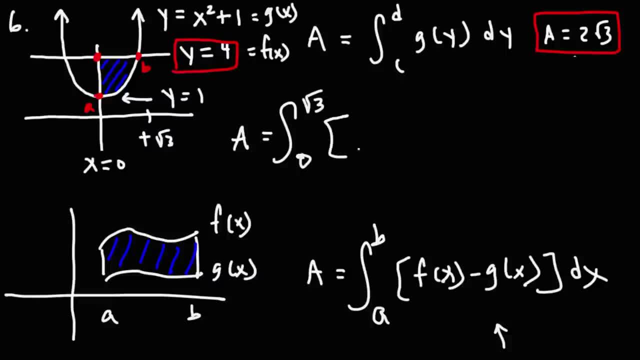 a is 0.. b is the square root of 3.. And then f is 4 minus g, which is x squared plus 1.. So we could simplify this expression: 4 minus 1 is 3.. So this simplifies to 3 minus x squared if we distribute the negative sign. 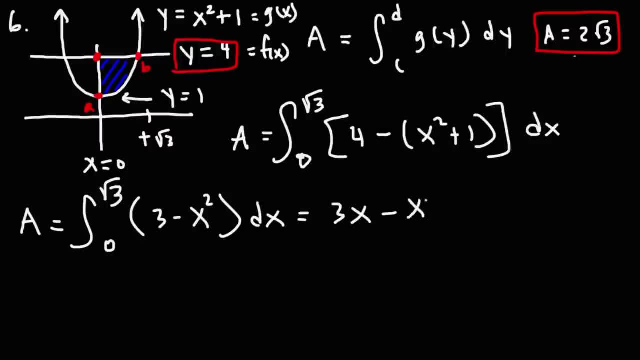 Anti-derivative of 3 is 3x For x squared, it's going to be x cubed over 3, evaluated from 0 to root 3.. So plugging in root 3, we have 3 times root 3 minus root 3 to the third power over 3.. 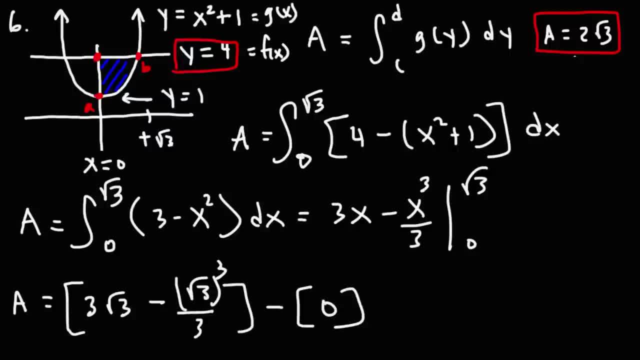 And all of that Minus 0.. So root 3 to the third power. So basically we have it 3 times. If we multiply the square root of 3 times the square root of 3, we're going to get the square root. 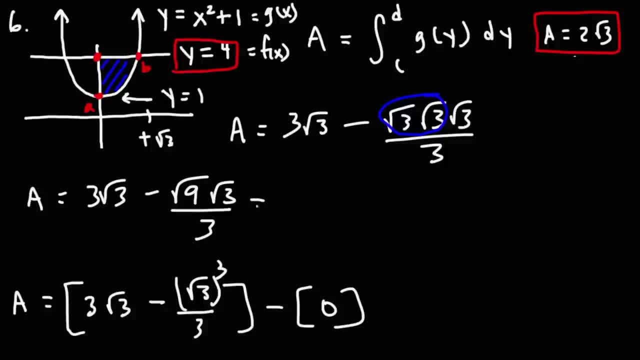 Of 9.. And the square root of 9 is 3.. So we have this, And 3 divided by 3 is 1.. So we have 3 square root, 3 minus 1 square root 3.. And 3 minus 1 is 2.. 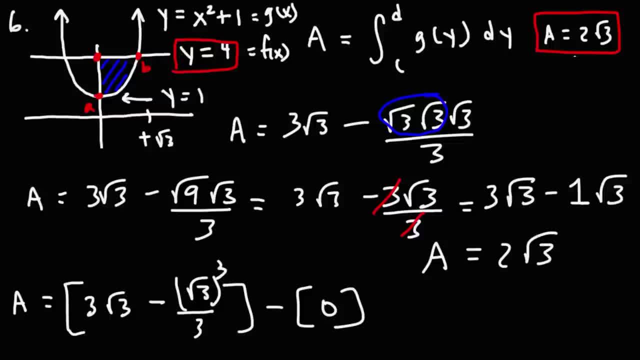 So we get: the area is 2 square root 3.. So those are two ways in which you can calculate The area of the shaded region. You can do it in terms of x or you can do it in terms of y, Depending on how you want to set up the problem. 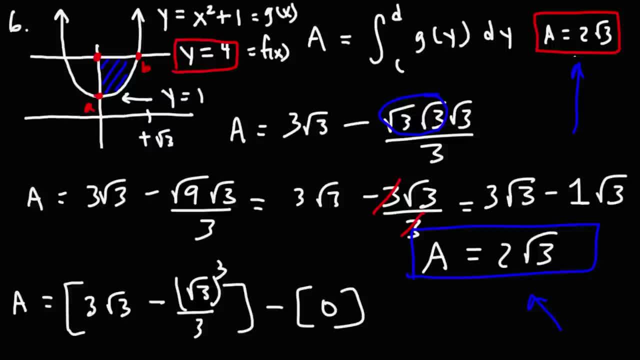 Just remember: if you do it in terms of x, you need to use a and b, which are x values. If you do it in terms of y, you need to use c and d, which are y values.